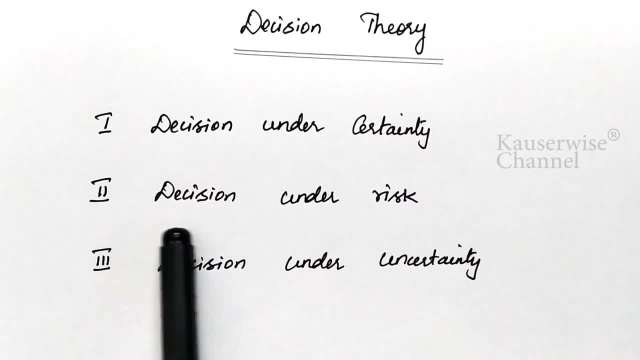 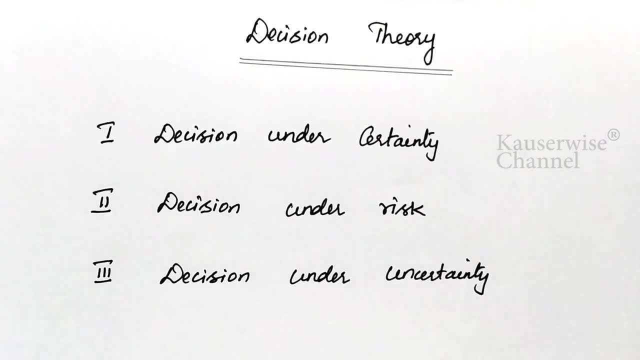 Okay. so unfortunately, the environment of information is limited, So it is known as ーン environment. Then the information taken is measured by is overwhelm of information. The information is then just providing parameters based on the information. the same way, user information buildsshots, video, video, digital pictures, then we can call them as decision. 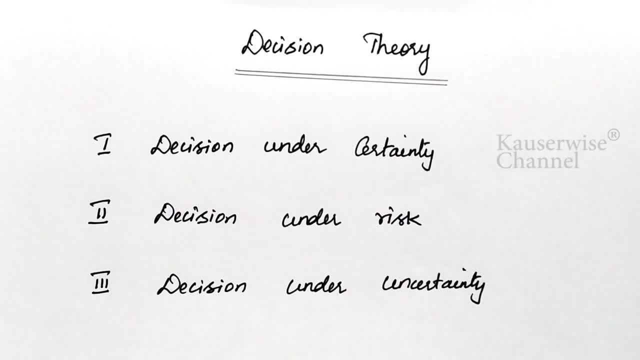 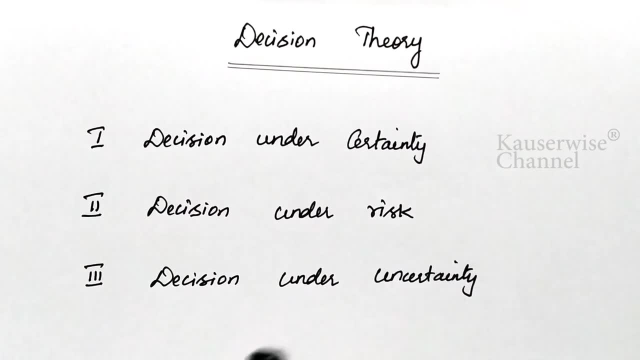 environment. So in this situation again, ID is both of these behaviors. Uh, so what should seems like an interesting way of saying: Since全部 data, do we want data sets, in this case probability distribution. Okay, so this kind of decision is called decision under risk, Okay, 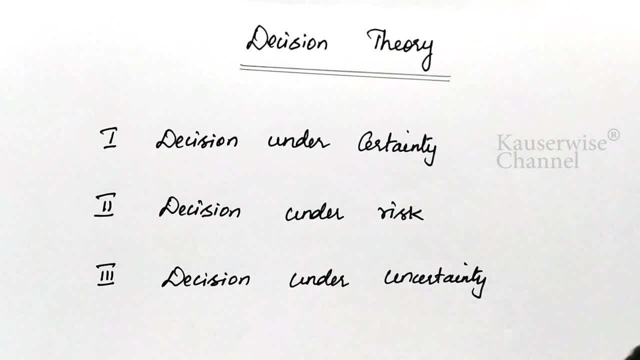 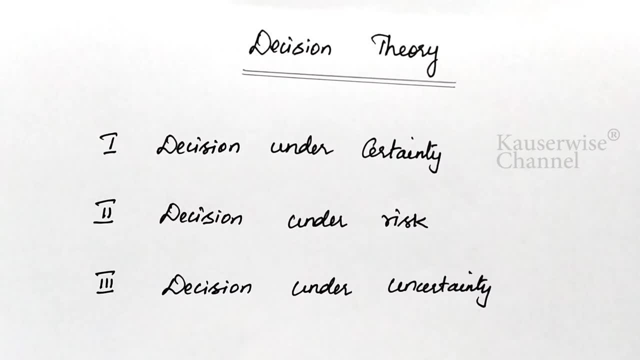 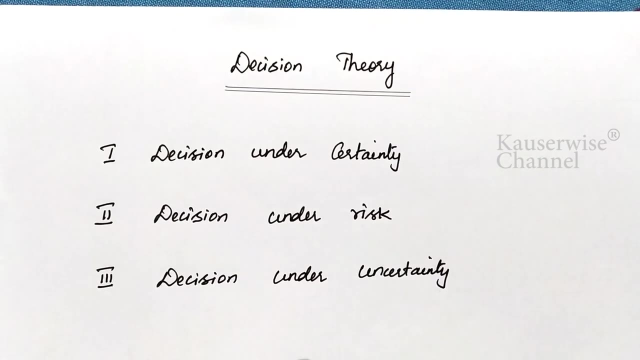 the third one is decision under uncertainty. See here: if the availability of information for a decision environment is incomplete, okay, then the decision taken under such an environment is called decision under uncertainty. Under this environment, there are five criteria. are there to make a? 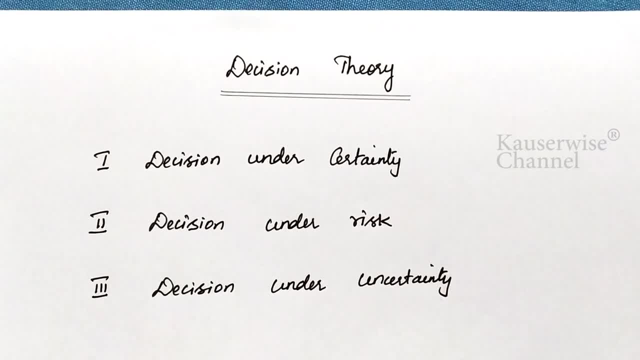 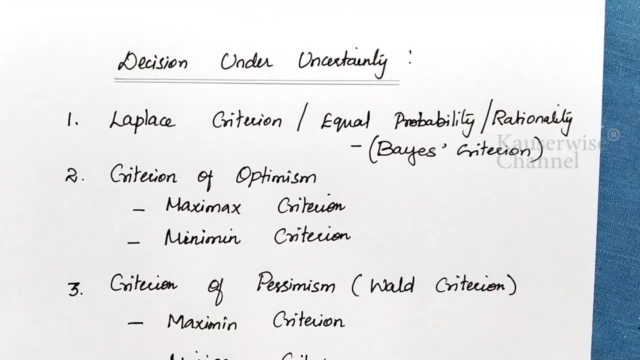 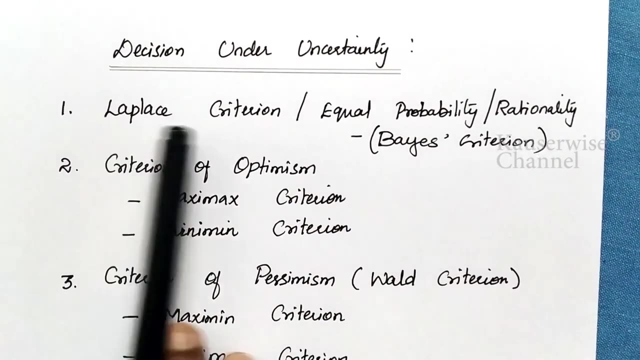 decision. So in this video we will see the problem for decision under uncertainty. Okay, first let us see the five criteria under this environment. Now let us see five criterion which comes under uncertainty. Okay, see, the first one is Laplace criterion, otherwise called as: 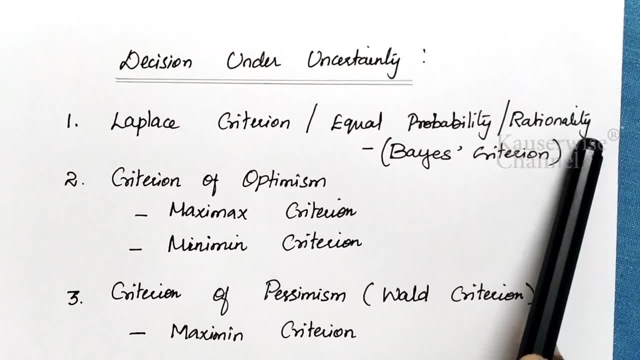 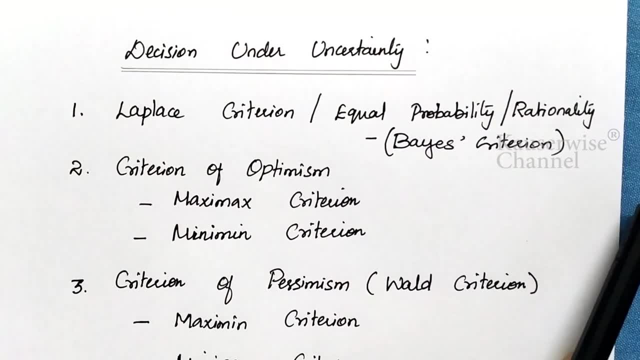 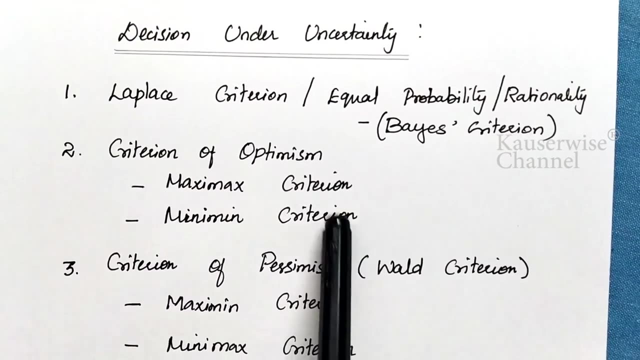 equal probability, or rationality or Bayes criterion- These are the other names for Laplace criterion- Okay. the second one is criterion of optimism. Okay, so under this optimism criterion we have two sub criteria. The first one is MaxiMax criterion and the other one is Minimin. 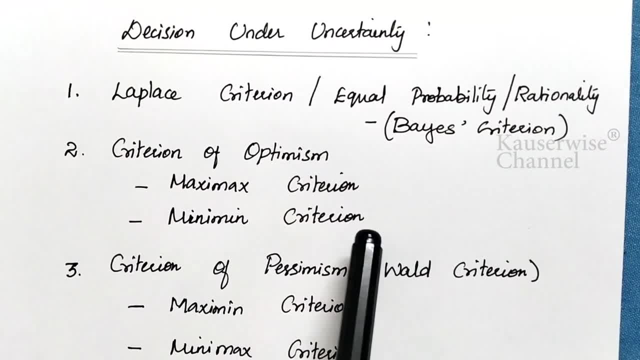 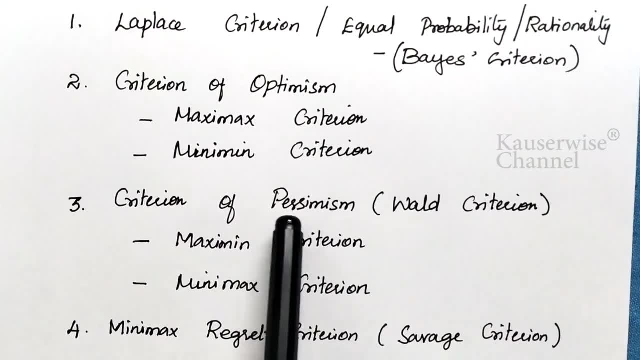 criterion. These are the two different types of criterion which comes under optimism: Okay, and the third one is criterion of pessimism, otherwise called as Wald criterion. So here also we have two different types. Okay, so under this criterion we have two sub criteria under optimism. Okay, so under the 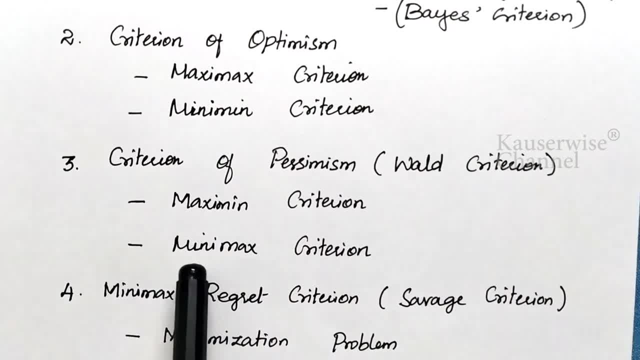 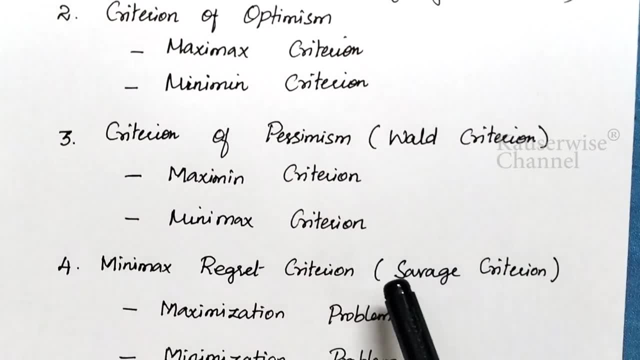 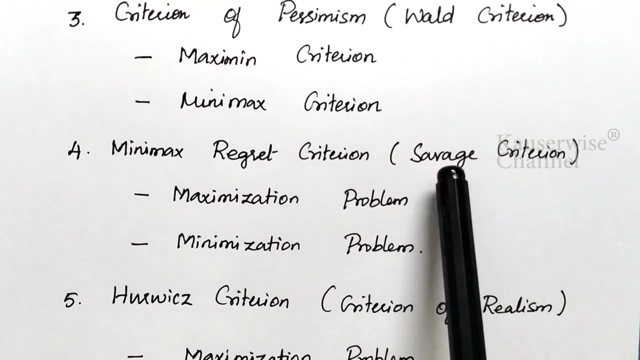 one is maximin criterion, the another one is minimax criterion. so these are the two types of criterion which comes under pessimism, okay, and the next one is minimax regret criterion, otherwise called a save age criterion. so here also we have two different types. the first one for maximization, 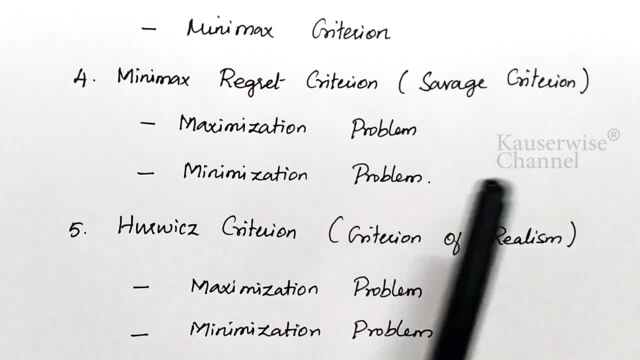 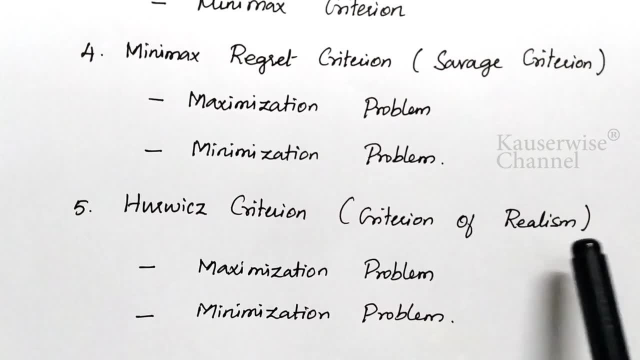 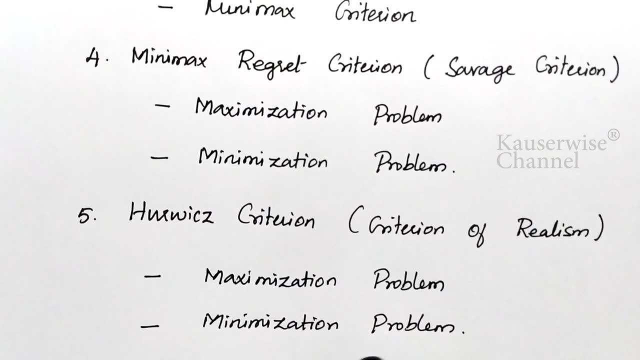 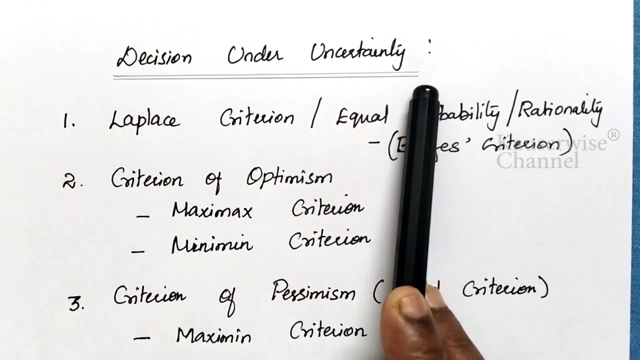 problem, the another one for minimization problem. okay. and the last one is horwich criterion, otherwise called as criterion of realism. okay. again, it has two different types: the first one for maximization problem, the another one for minimization problem. these are the five criterion which comes under decision and uncertainty. okay, now we are going to see the problem for each and. 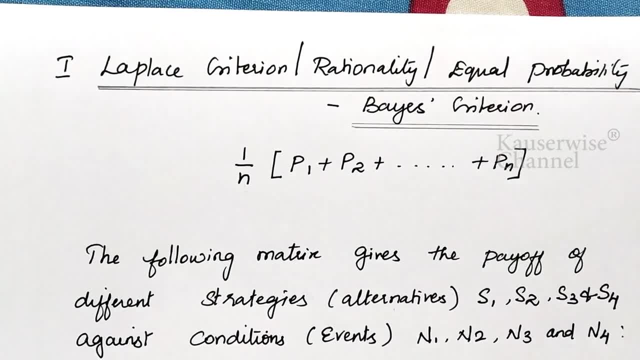 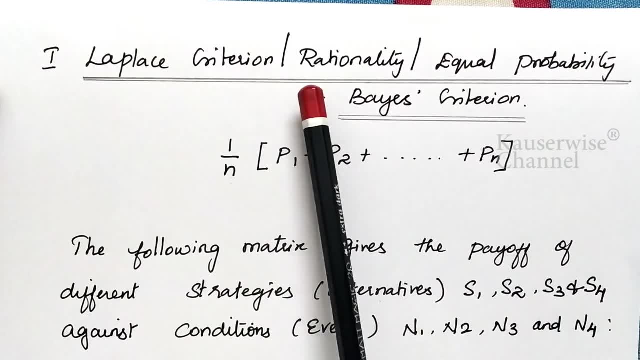 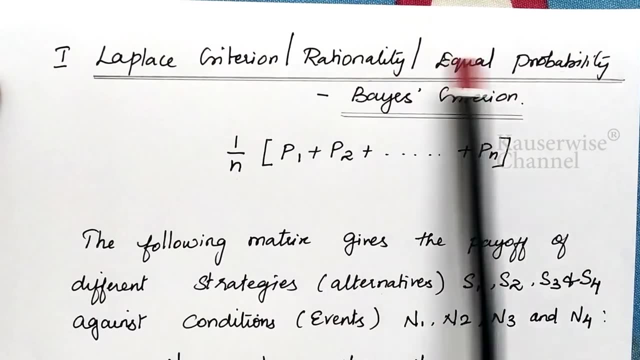 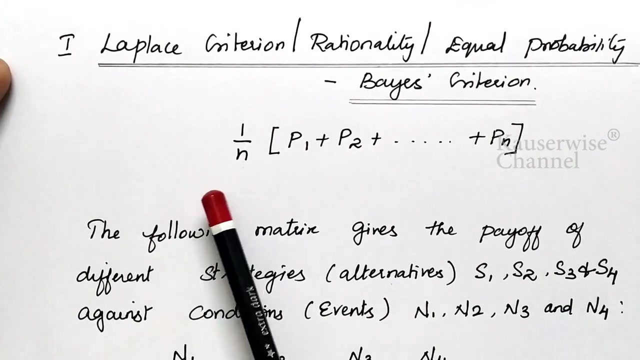 every criterion separately. now let us see the first criterion under uncertainty. okay, the first one is laplace criterion, otherwise called as rationality or equal probability or base criterion- these are the other names for laplace criterion. okay, so here. first you need to find out the expected value. 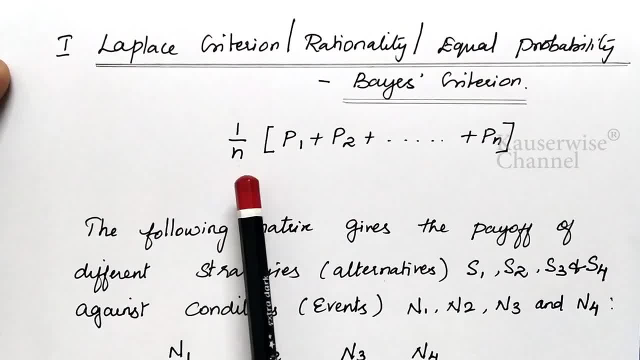 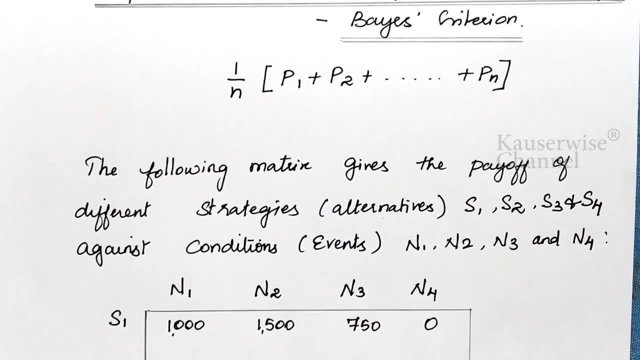 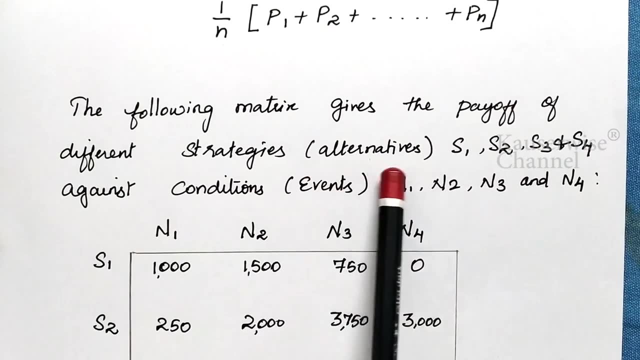 for each and every strategies. okay, see, this is the formula. i will explain this formula along with the problem. okay, now let us see the problem. for laplace criterion. see the following matrix gives the payoff of different strategies, that is, alternatives s1, s2, s3 and s4. okay, against conditions. 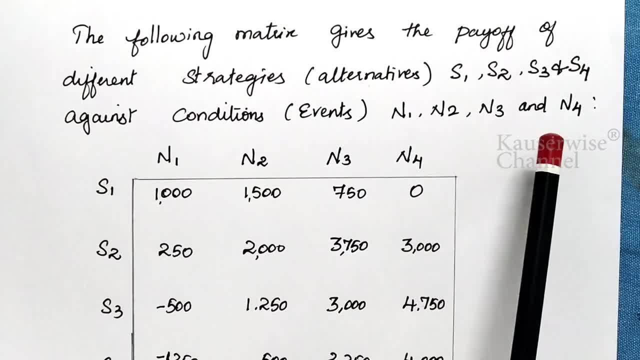 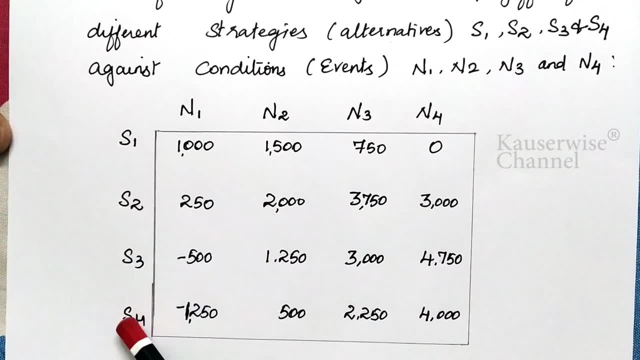 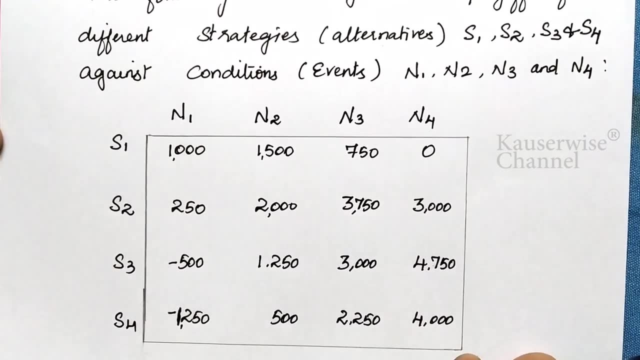 that is, events n1, n2, n3 and n4. so this is the payoff matrix. here we have four alternatives, four strategies are there and four events, four conditions are there. okay, now, with this available payoff matrix, you have to select the payoff matrix and you have to select the payoff matrix. 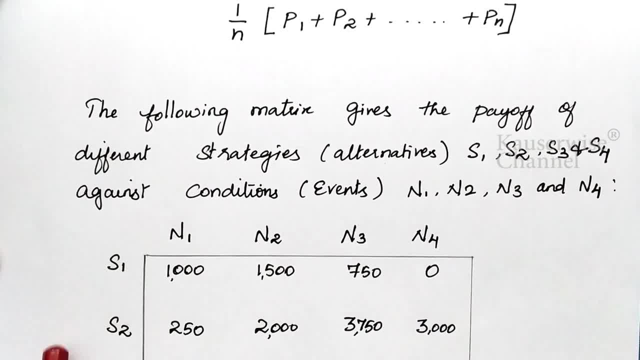 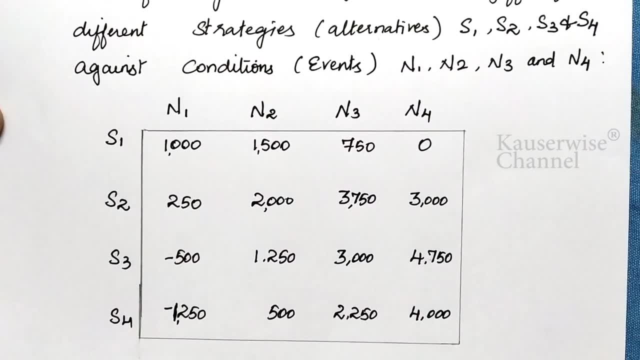 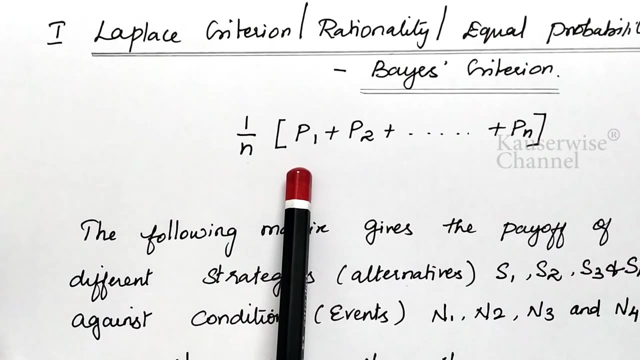 with the best alternative, that is, you have to select the best strategies. so we have four strategies, no, so first you have to apply the formula to find out the expected value for each and every strategy by using this formula to find out the best decision. okay, first we need to find: 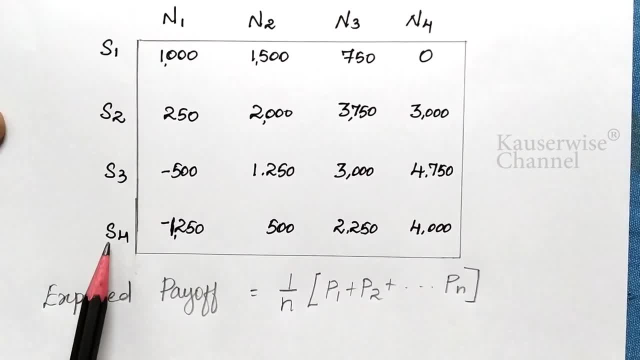 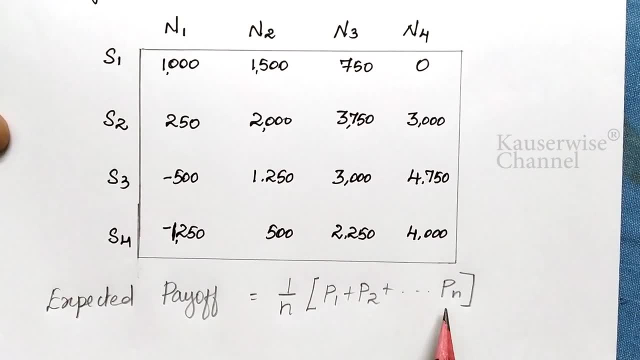 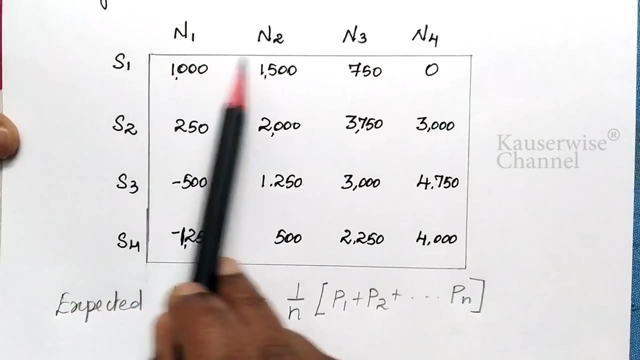 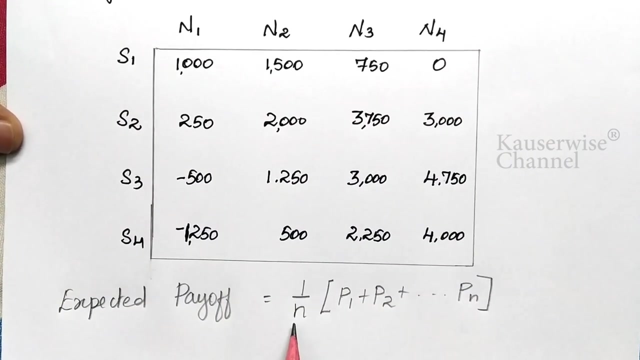 out expected payoff for each and every alternatives by using the formula. the formula is 1 by n into p1, p2 till pn. see n represent number of events. okay, for the first strategy. how many events are there? n1, n2, n3, n4. four events are there: no, so n represent number of events. okay, and p1, p2, p3 represent 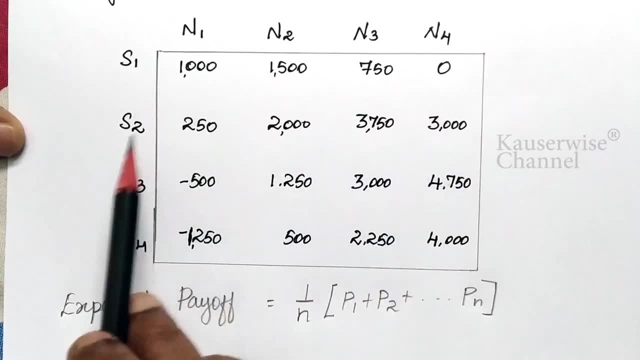 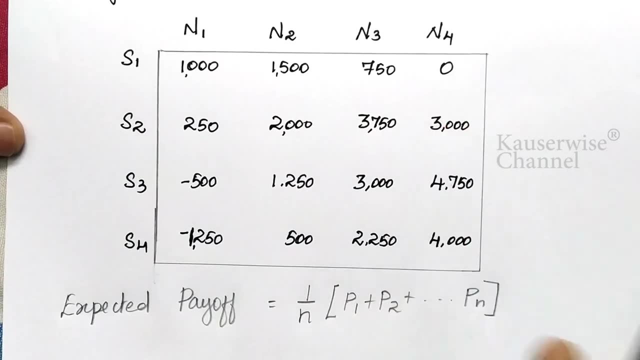 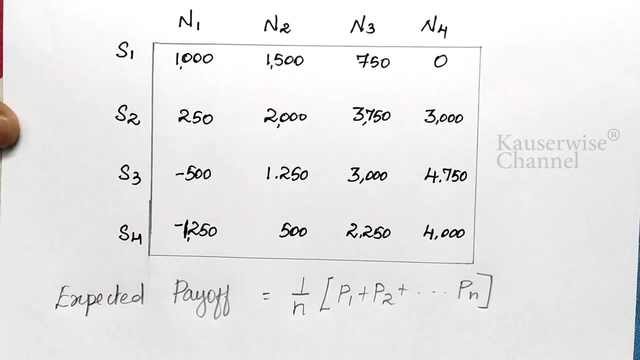 the payoff value of each and every alternatives. for the first alternative, these are the p values, that is, p1, p2, p3 and p4. okay, now we have to apply the formula to find out the expected payoff for each and every alternative separately. i'll show the calculation for the first one first. 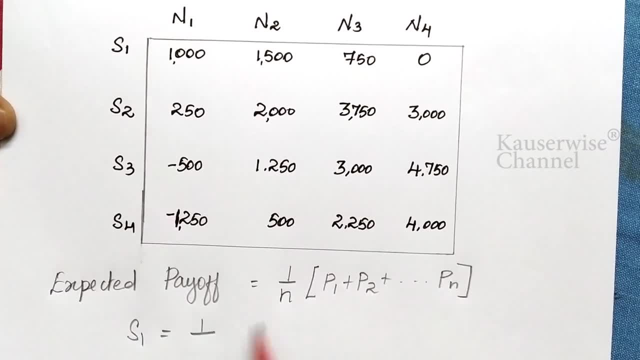 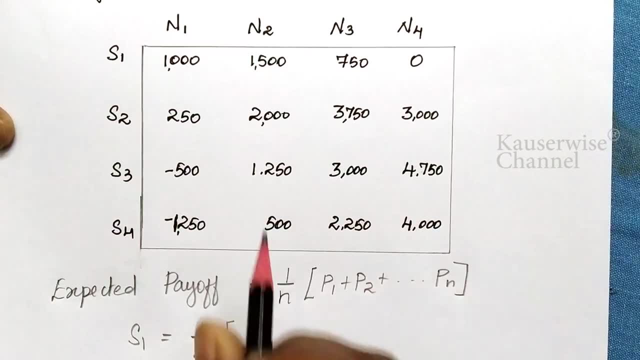 alternative is: s1 is equal to 1 by n represent number of events. here we have four events, no, so 1 by 4 into. for the first alternative, p1 is thousand, p2: thousand five hundred, p3, seven. fifty agency: we have four things now we have four times. we have four events, so we have four times. 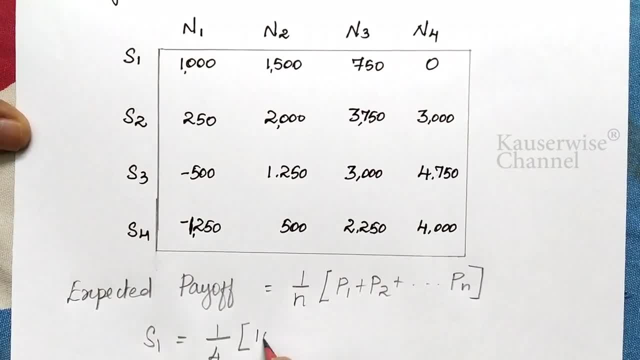 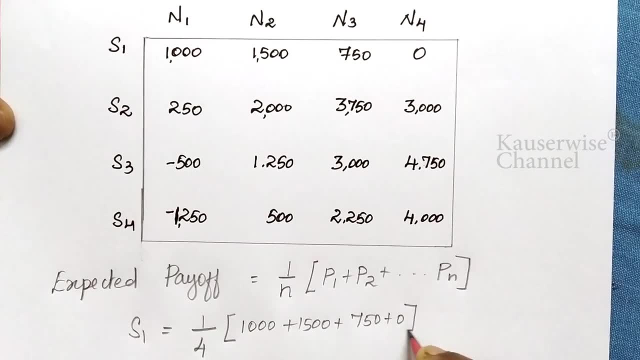 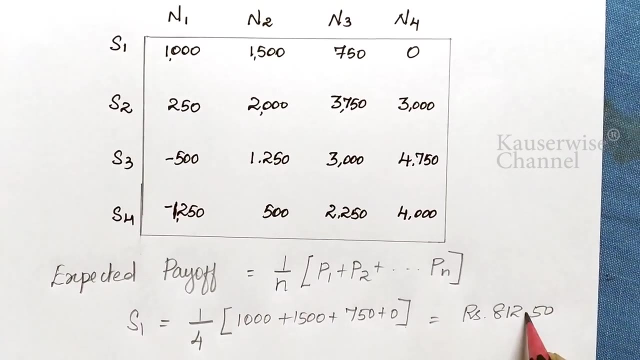 p for 0. so just add 1000 plus 1500 plus 750 plus 0. okay, you will be getting rupees 812, 50 pies: 812 rupees 50 pies. so this is the expected payoff for the first alternative. okay, in the same way. 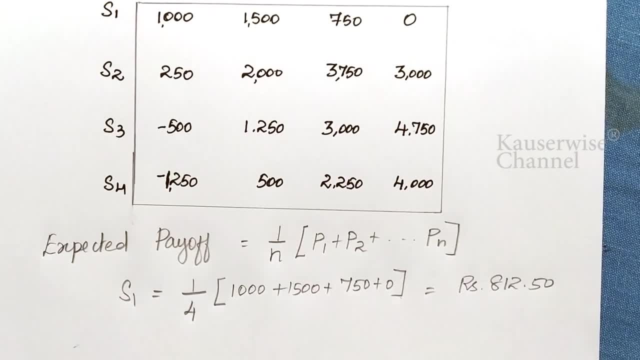 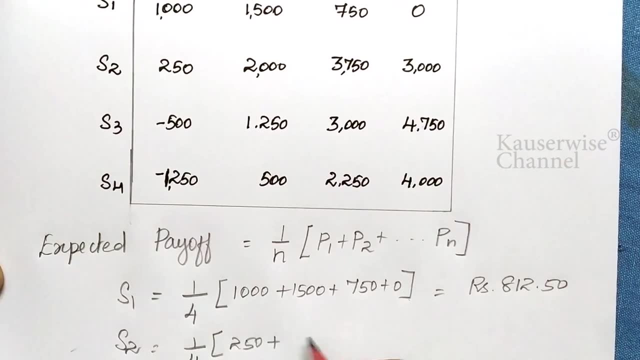 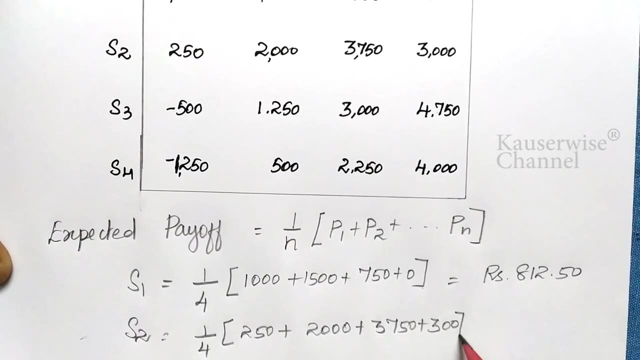 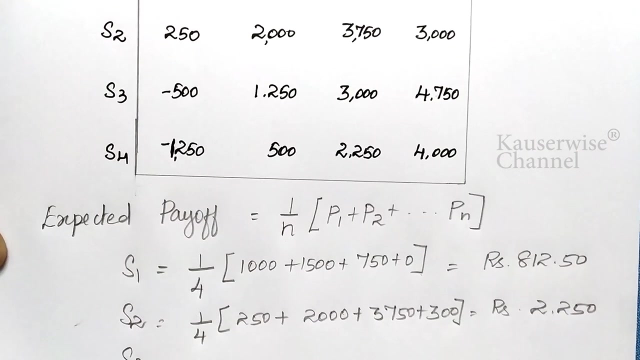 you have to find out the expected payoff for s2, s3 and s4. for s2, 1 by 4 into 250 plus 2000 plus 3750 plus 3000. answer is rupees 2250. in the same way for s3, 1 by 4 into minus 500. 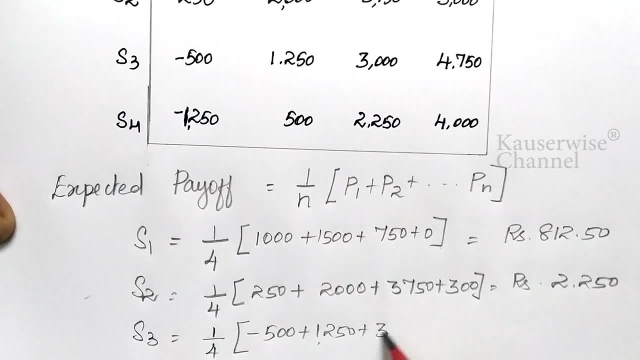 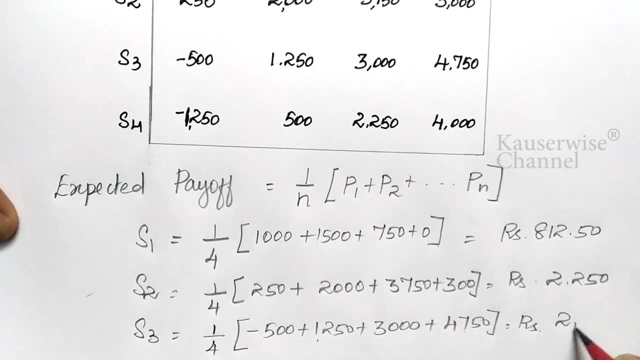 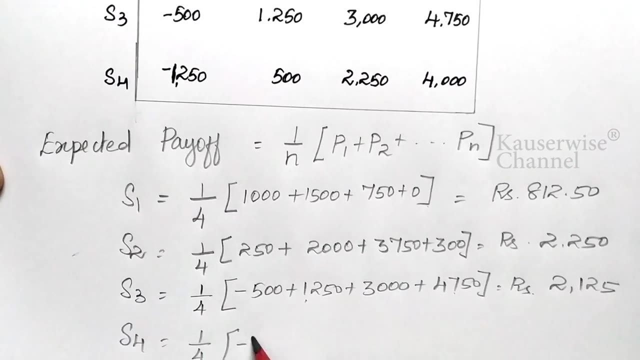 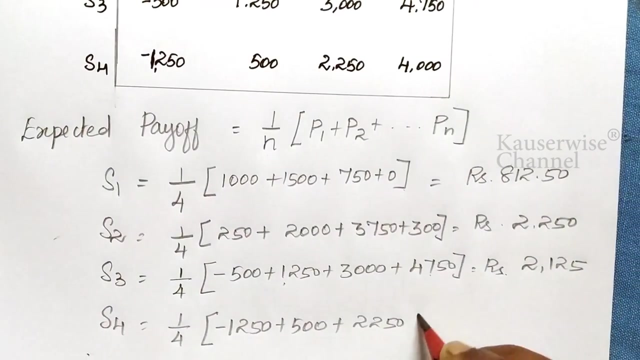 plus 1250 plus 3000 plus 4750, you will be getting rupees 2125 for s4. 1 by 4 into minus 1250 plus 500 plus 2250 plus 4000, you will be getting rupees. 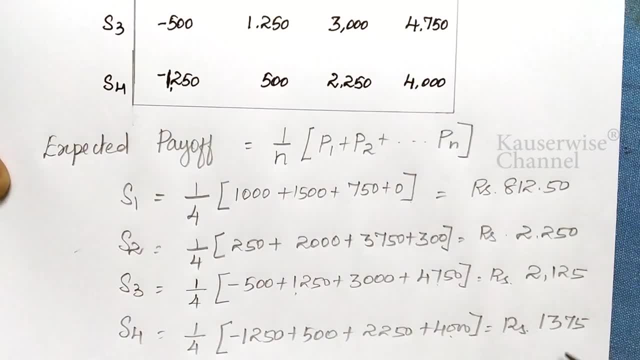 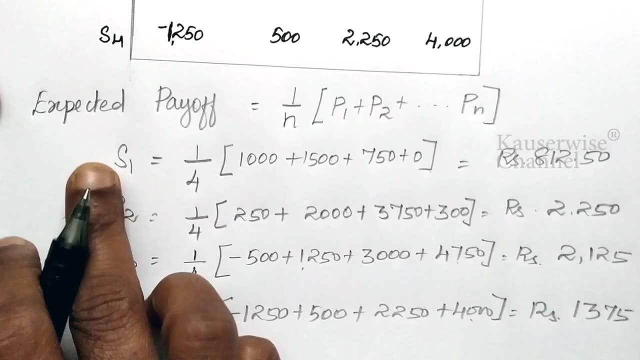 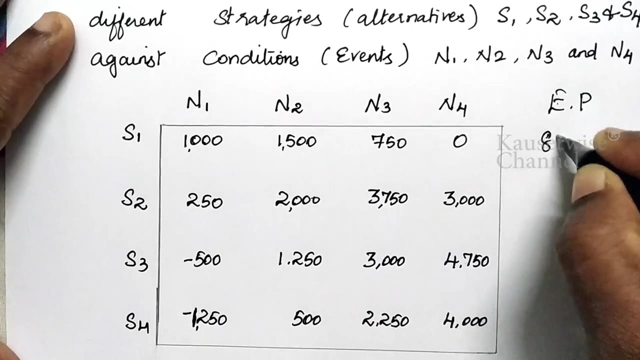 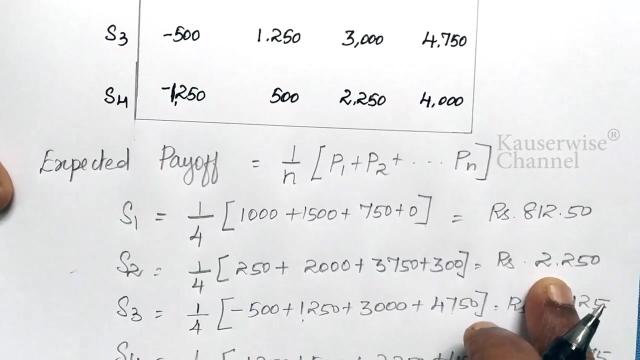 375. okay, these are the expected payoff for each and every alternatives. now you can enter the value in the respective alternatives, see: the expected payoff for the first alternative is 812.5. okay, for the second alternative, the expected payoff is 2250. okay, for s2, s3 and s4, you will be getting rupees 2250 plus 3000 plus 3000. okay, these are the expected. 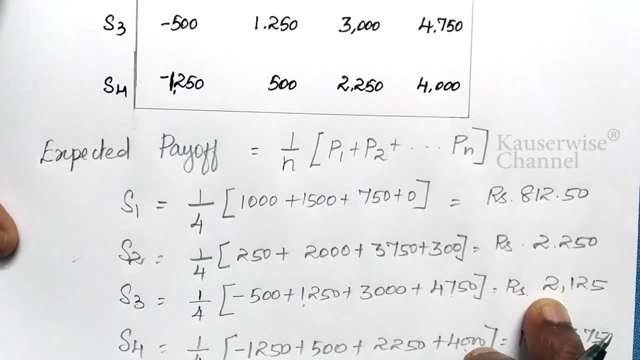 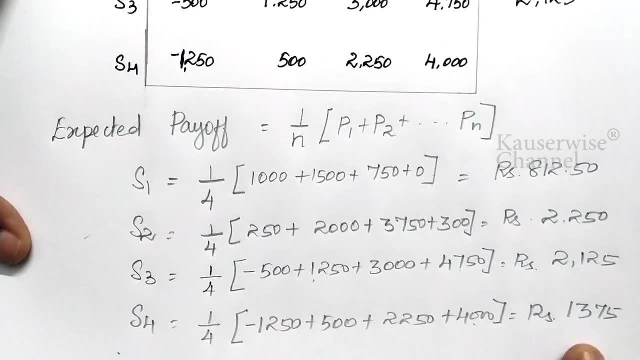 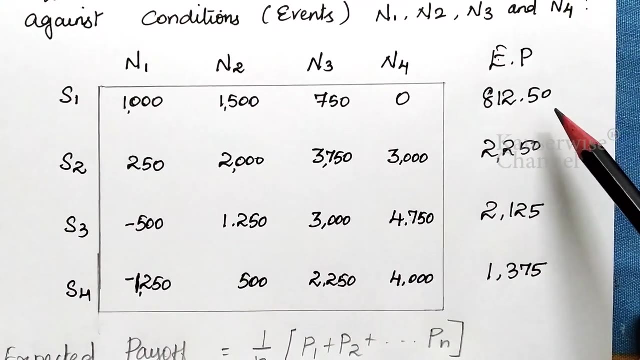 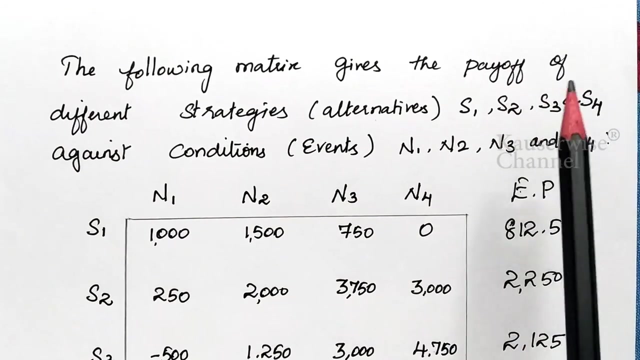 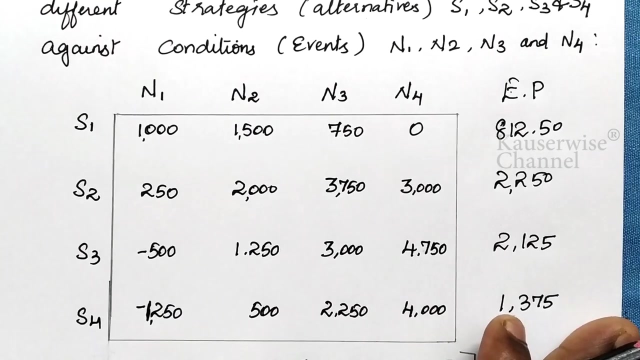 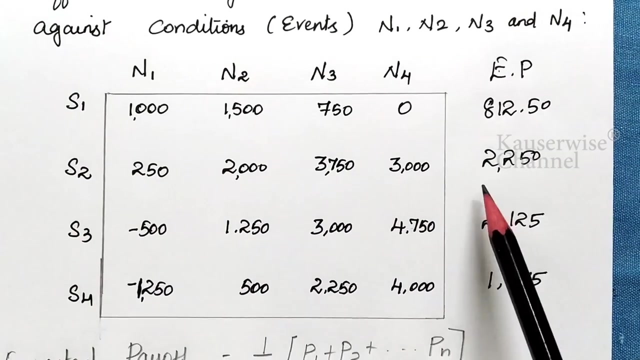 payoff for s3, alternative 3, is the value 2125, for the fourth alternative, 1375. now we have calculated expected payoff for four alternatives. okay, now see the problem, since the problem is payoff matrix, so we need to select the maximum expected payoff. see see the payoff matrix. for the first alternative, expected profit is 812.5. for s2: 2250. 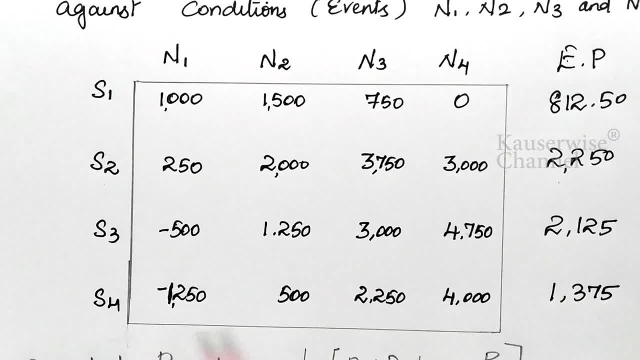 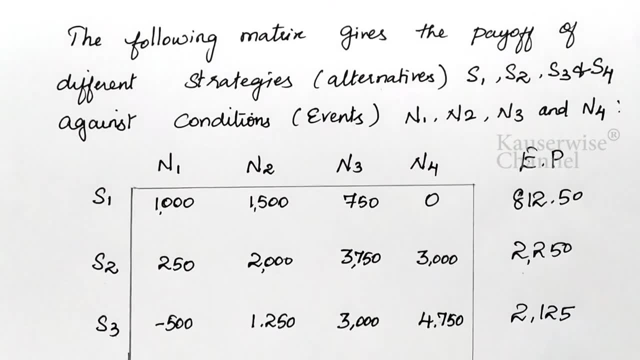 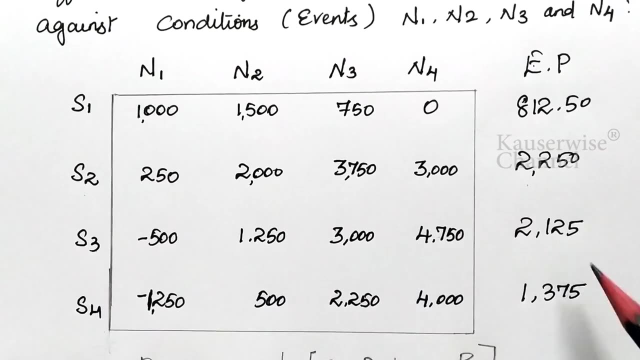 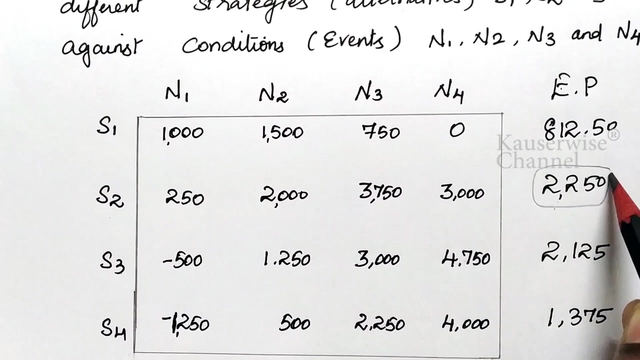 for s3 2125. for s4 1375. now, since this is the payoff matrix, you have to select the maximum expected payoff. which one is highest value: 812, 2250, 2125, 1375. so 2250 is the highest value. so now we have to select. this one, that is, s2, is the best alternative. we 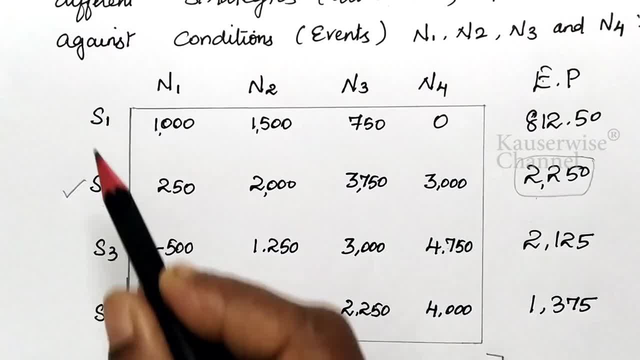 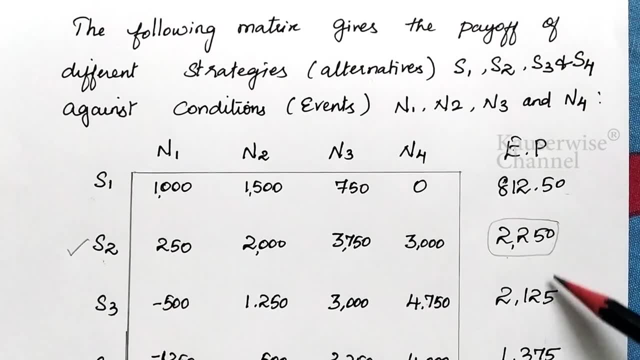 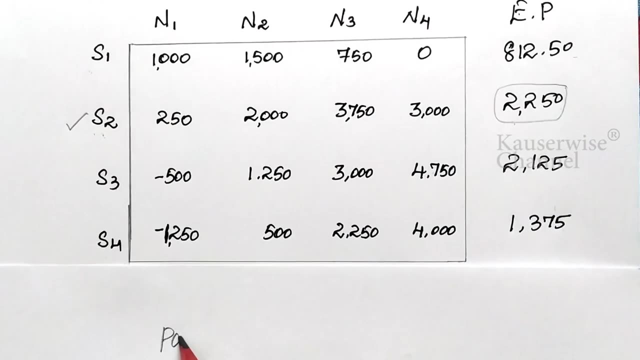 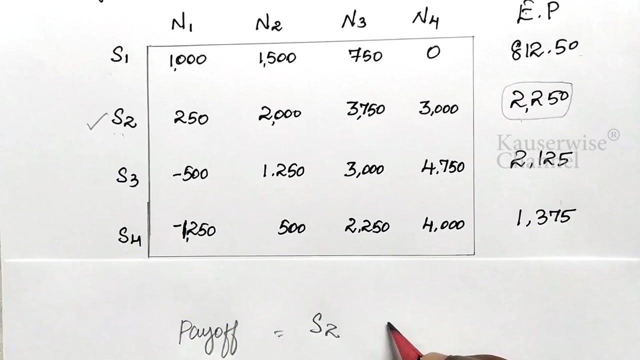 are going to select s2 as the best alternative among the four alternatives. see, since the problem is payoff matrix, we need to select the maximum expected payoff. which one is maximum value. s2 is the maximum value. so for payoff matrix, s2 gives the maximum expected payoff, that is, 2250. okay, 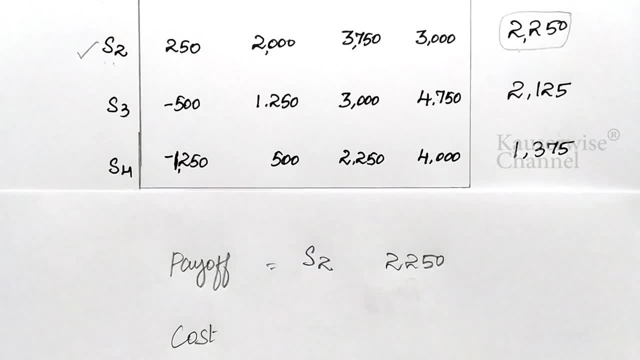 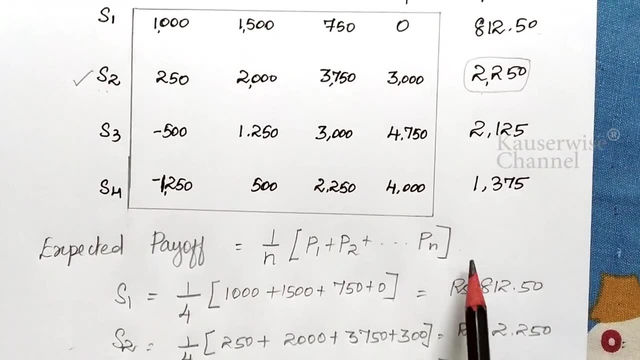 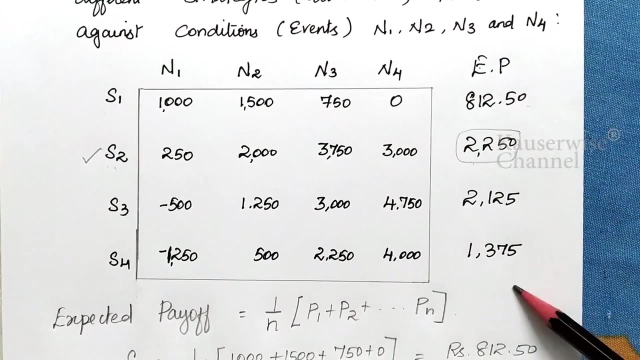 in case of cost matrix, say, in case of cost matrix instead of payoff matrix, you need to apply the same formula to find out the value for each and every alternatives. then you have to select the least value. okay, which one is least value and which one is least value? so in case of cost matrix, 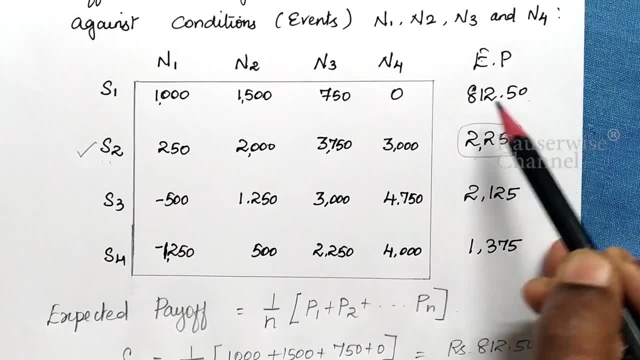 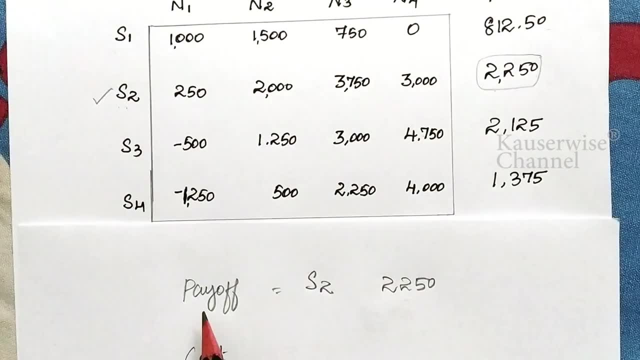 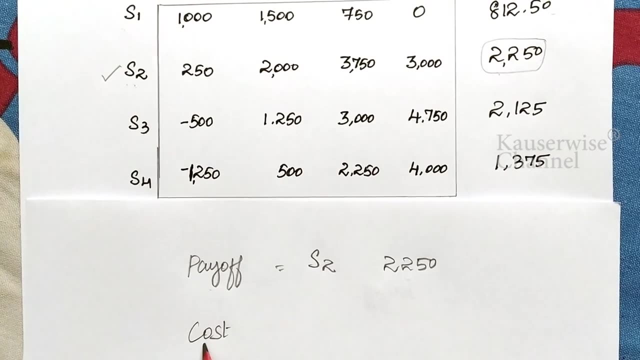 least value. 812.5 is the least value. okay, you have to select S1 as the best alternative out of four other alternatives. okay, so for payoff matrix, you have to select the maximum value. so S2 gives the maximum benefit. in case of cost matrix, you have to select the minimum value. 812.5 is the minimum. 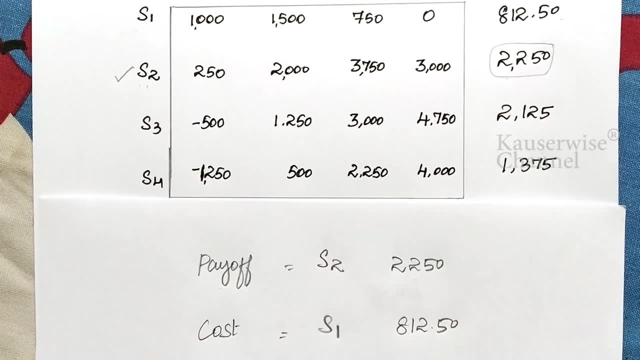 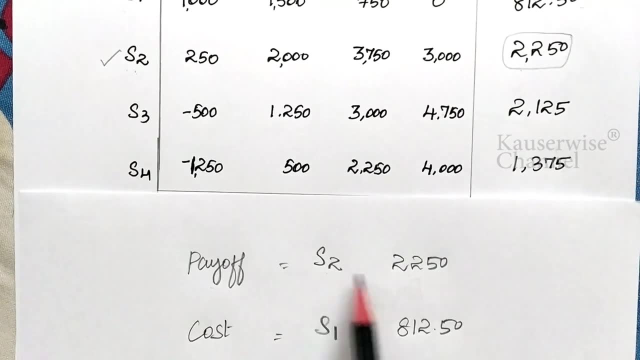 value no. so S1 is the best alternative out of four alternatives. so for the cost matrix, you have to select based on minimum value. for payoff matrix, you have to select based on the maximum value according to the problem. you have to take a decision. this is the way to take a decision. 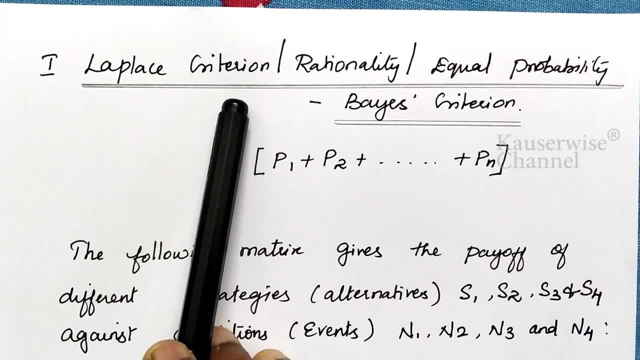 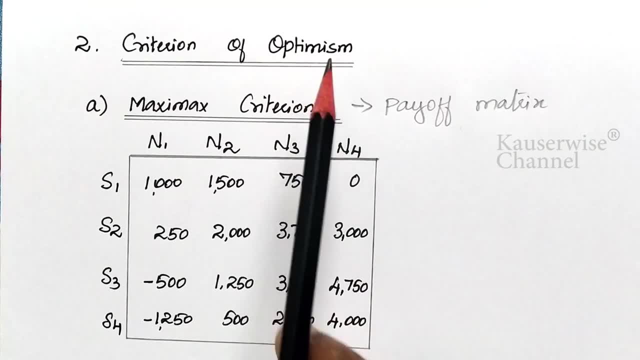 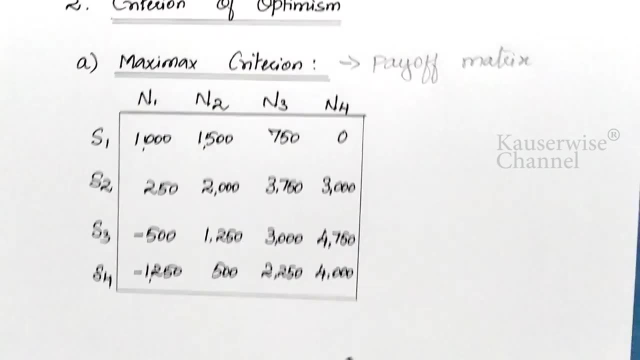 under Laplace criterion. now let us see the second criterion. look at the second one. the second criterion is criterion of optimism. in the optimism it has two subdivisions. the first one is maximax criterion, which is applicable for payoff matrix okay, and the second one is minimum criterion. 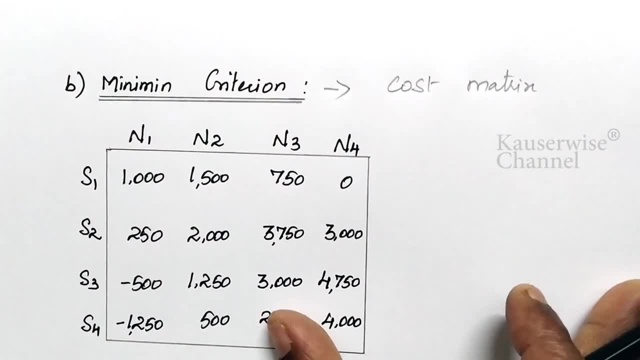 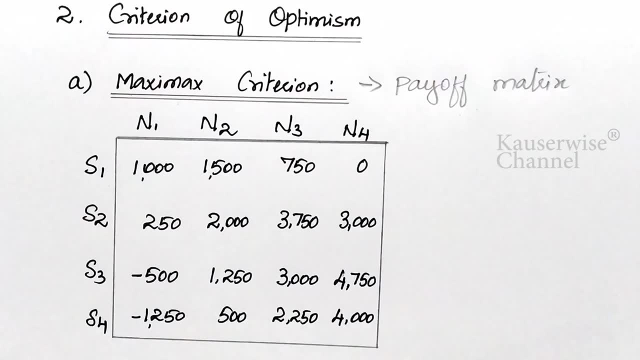 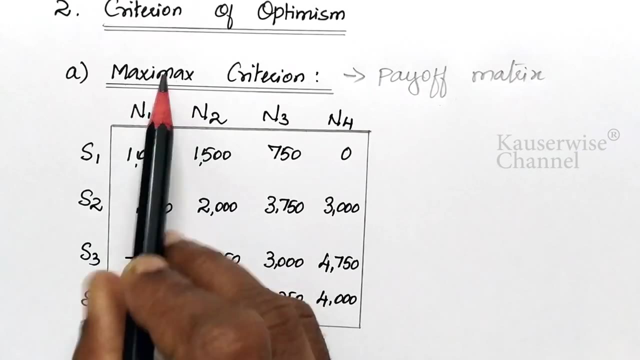 which is applicable for cost matrix. okay, now let us see the solution. how to find out the best alternative according to maximax and minimum criterion? look at the first one, according to maximax criterion. first you need to find out the maximum value for each and every alternatives. 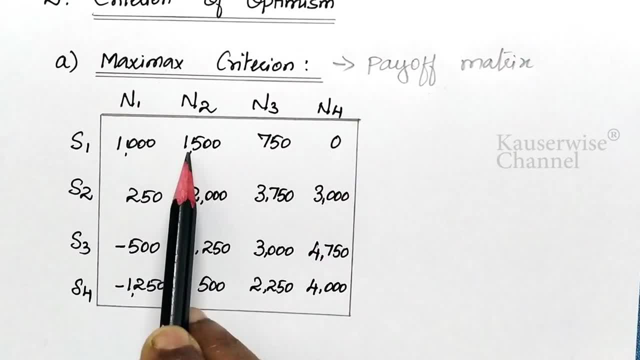 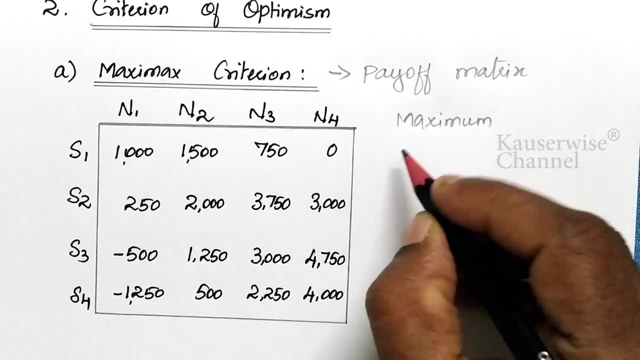 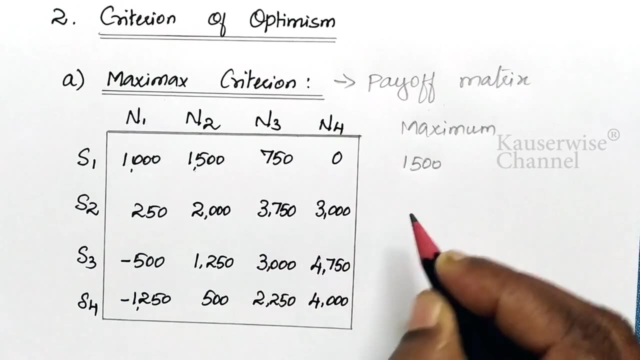 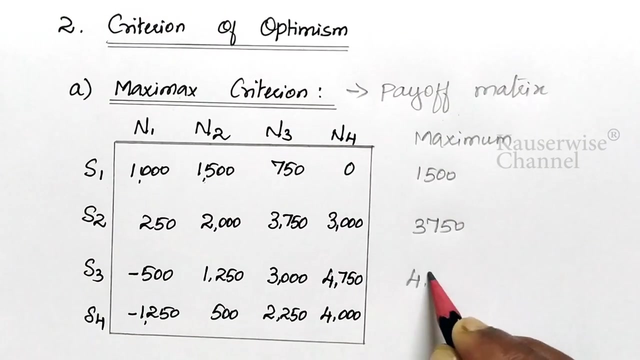 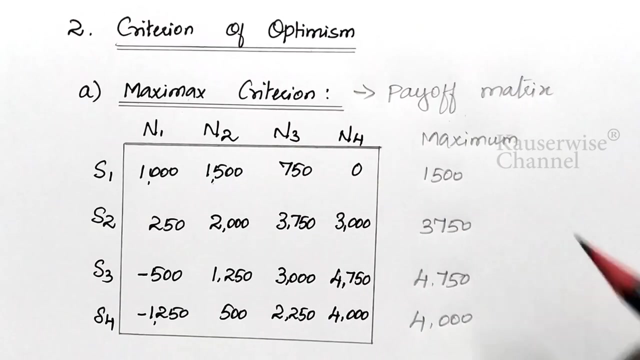 look at the first alternative, which is the maximum value: 1500. so first find out the maximum value for the first alternative, 1500. for the second alternative, which is the highest value, 3750. for the third alternative, highest value is 4750. for the fourth alternative, 4000 is the highest value. okay, after finding the maximum value for: 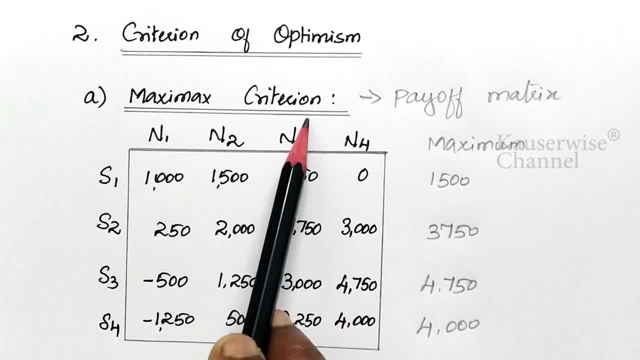 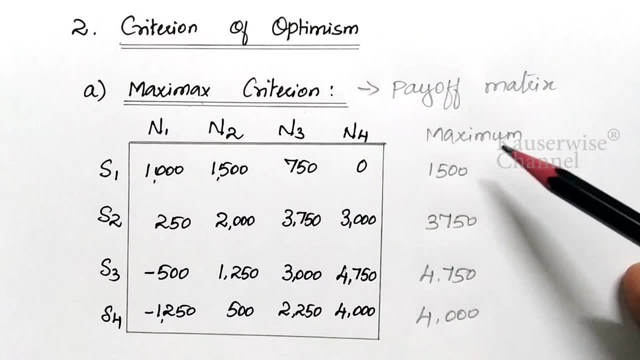 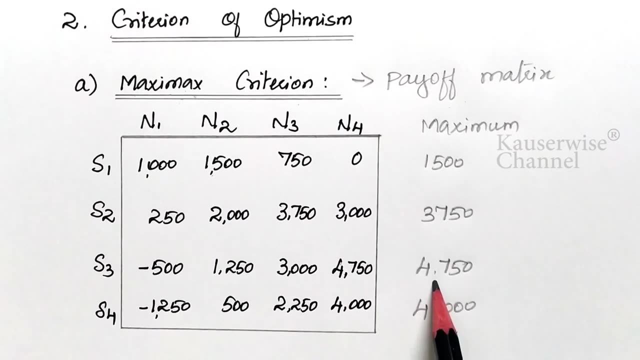 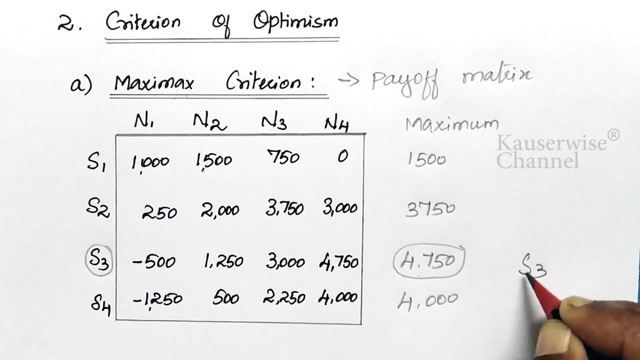 each and every alternatives according to maximax criterion, we need to select the maximum of the maximum value. so which is the maximum value out of the maximum values? so here, 4750 is the maximum of maximum payoff. so S3 is the best alternative to be selected for implementation. so S3 is to be. 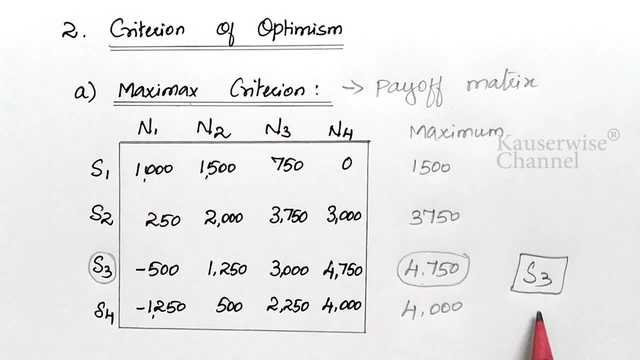 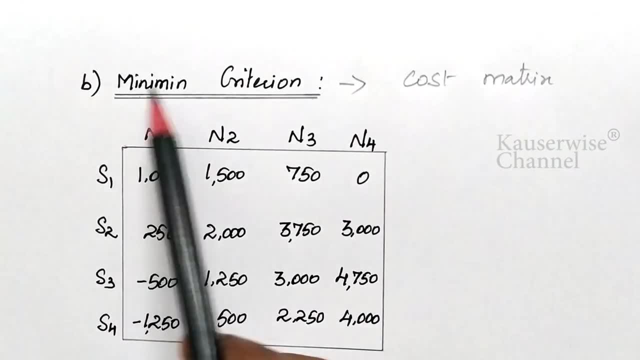 selected as a best alternative according to maximax criterion. now look at the minimum criterion. see according to minimum criterion. so this is applicable only for maximum value for each and every alternative, only for cost matrix. so here, first you need to find out the minimum value for each and. 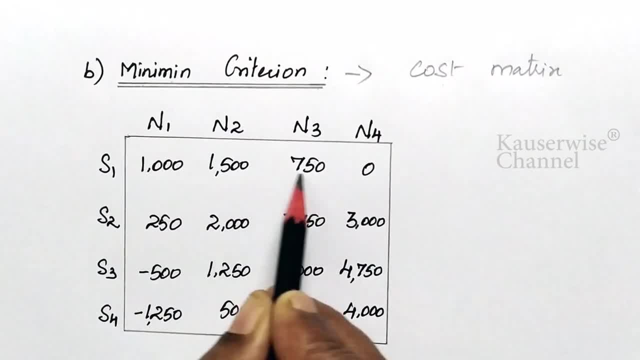 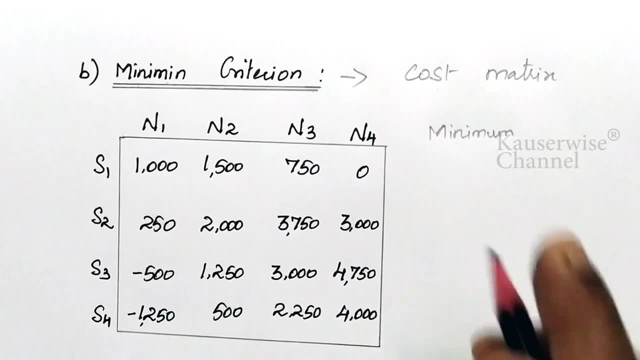 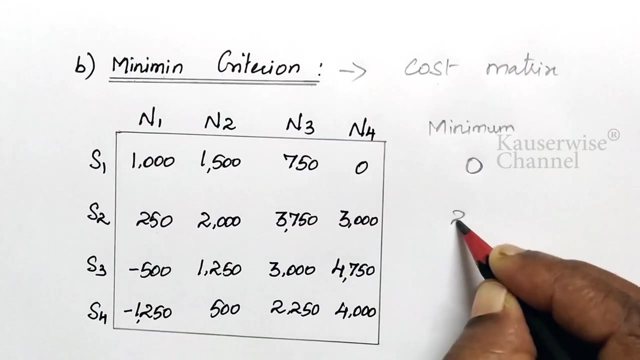 every alternative separately. look at the first alternative, which is the least value. 0 is the least value. so find out minimum value for each and every alternative. for the first one: 0. for the second alternative, 250 is the least value. for S3, which is the least value, minus 500 is the least. 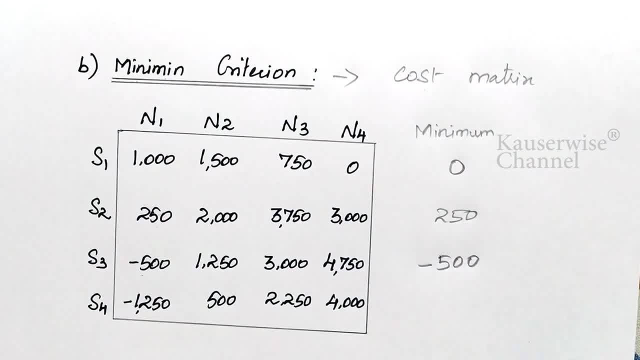 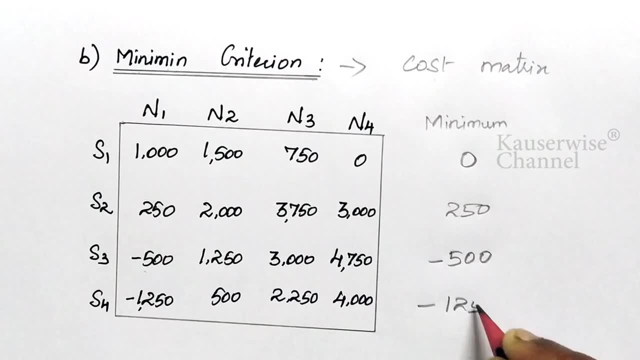 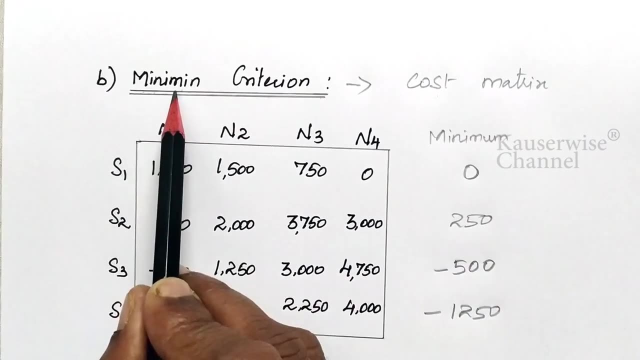 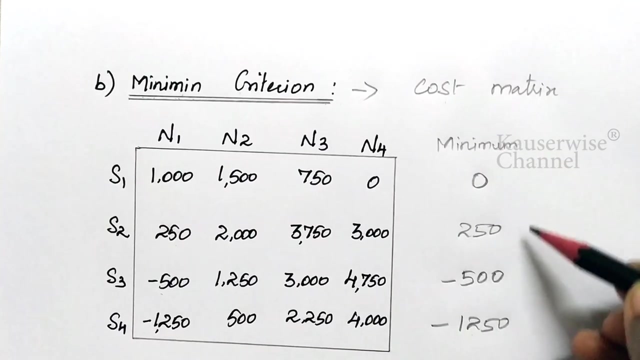 value for S4, which is the least value, minus 1250 is the least value. okay, so now you have to select the best alternative according to minimum criterion. so, according to minimum criterion, now you have to select the minimum of minimum values. so, out of the minimum values, which is the most minimum value? 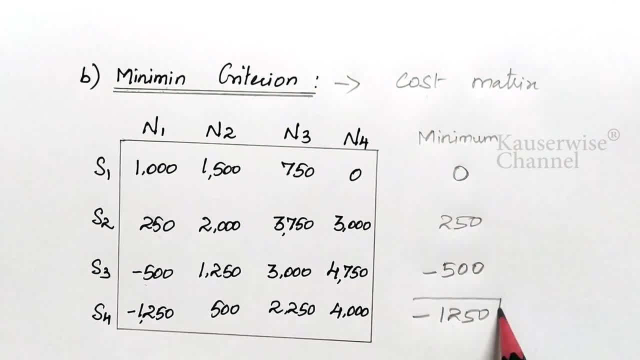 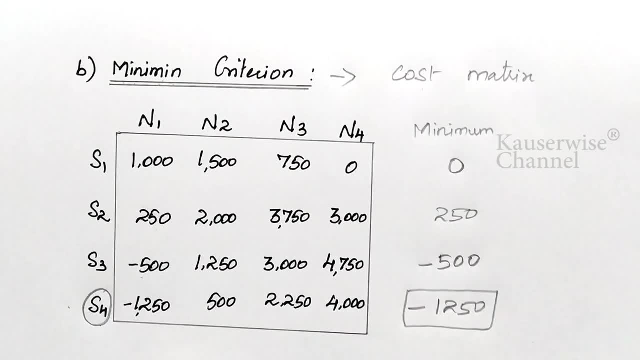 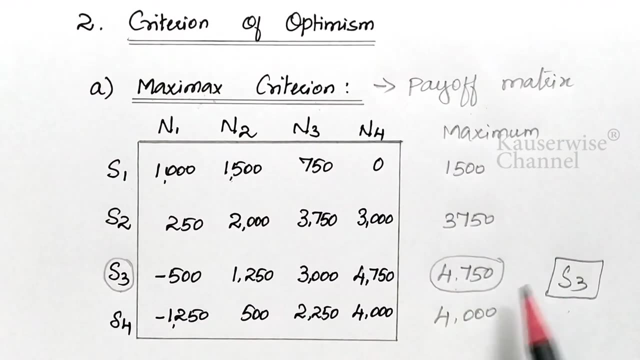 minus 1250 is the most minimum value out of the minimum values. so here first you need to find out the minimum values. so S4 will be selected as a best alternative according to minimum criterion. here, according to maximax criterion, we have selected maximum of maximum value. okay, according to. 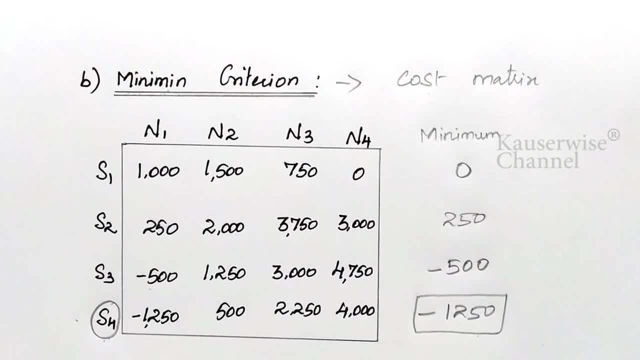 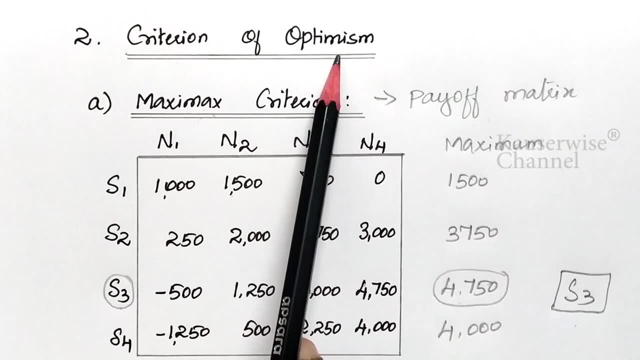 minimum. we have selected minimum of minimum values. okay, so these are the two sub criterion which comes under optimism. that is, criterion of optimism. now let us see the third one. so far, we have discussed two criteria, which are the minimum and the maximum values. so S4 will be selected as the 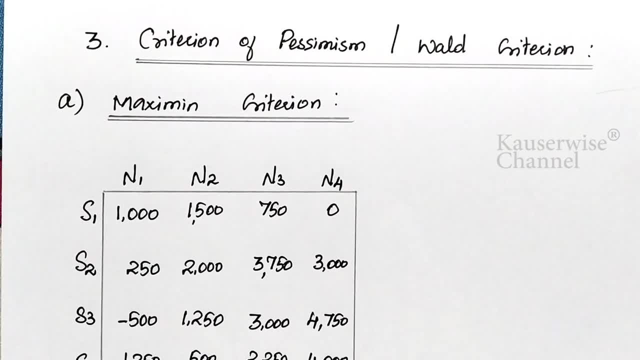 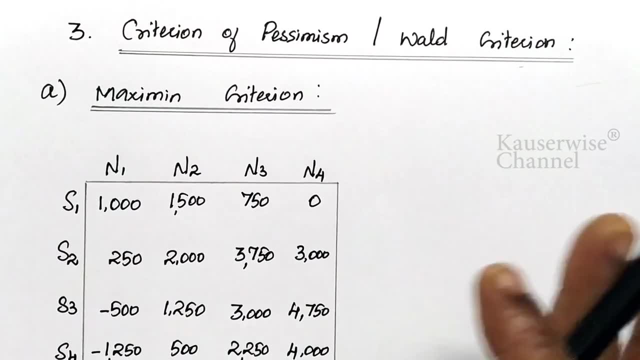 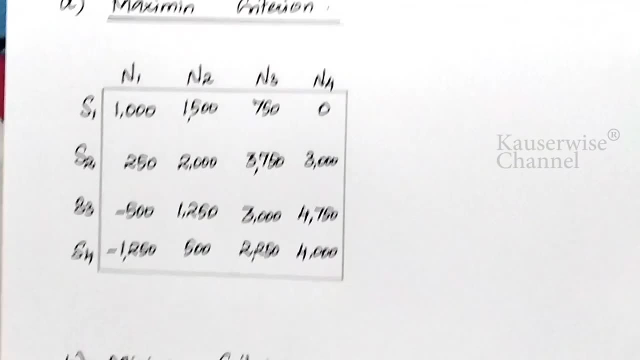 best alternative. according to minimum criterion, the first one is laplace and the second one is optimism. now let us see the third one, that is, criterion of pessimism or walled criterion. okay, according to pessimism, it has two subdivisions. the first one is maximum criterion, the second one 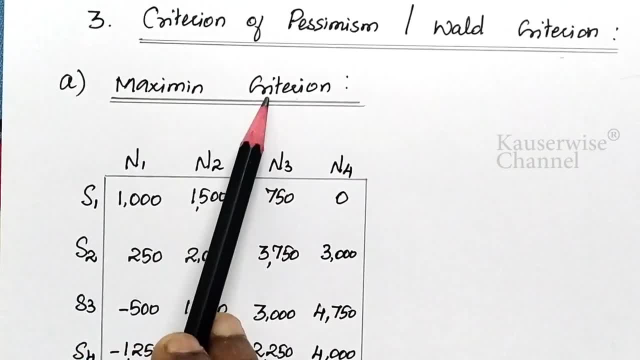 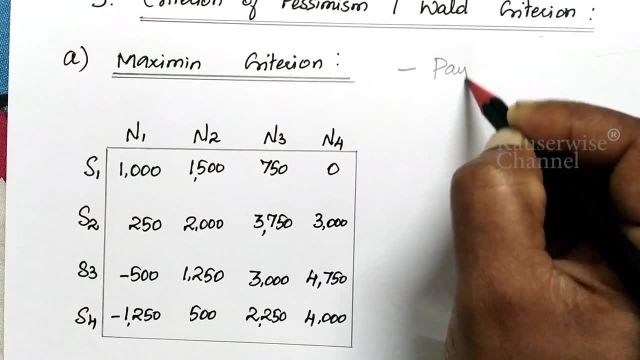 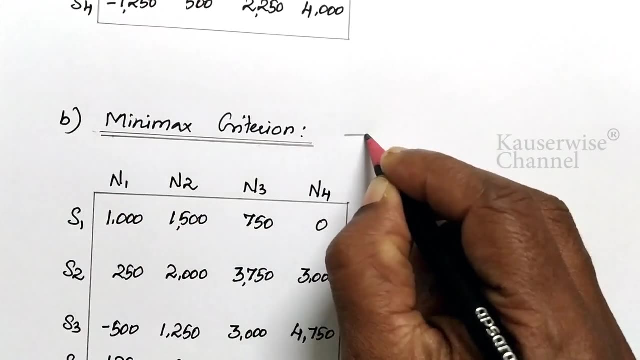 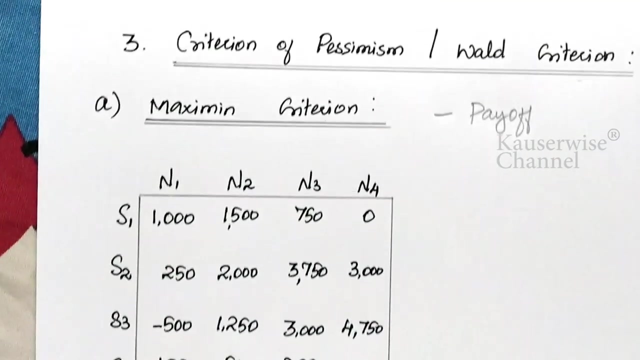 is minimax criterion see. the maximum criterion is applicable. the maxi value is there, no, so maximum is applicable for payoff matrix, okay. the second one is mini value is there now, so minimax criterion is applicable for cost matrix. okay. now let us see how to take a decision based on maxi, min and minimax. now let 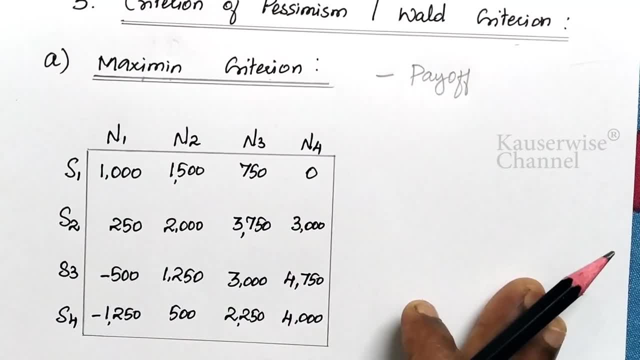 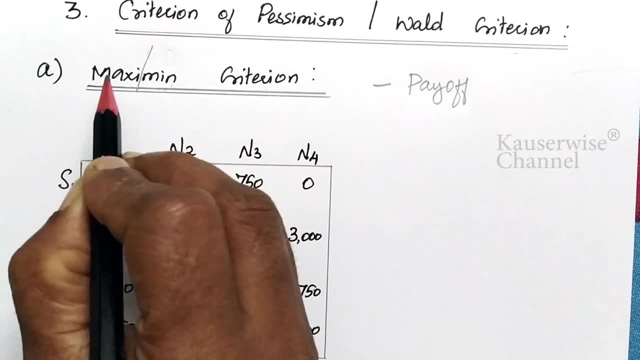 us see the first one, that is, maximum criterion. i'll tell you how to do this problem in a simple manner. just divide the term into two parts. that is, maxi, min. okay, first you have to do minimum, you have to find out the minimum values for each and every minimum value, and then you have to find out. 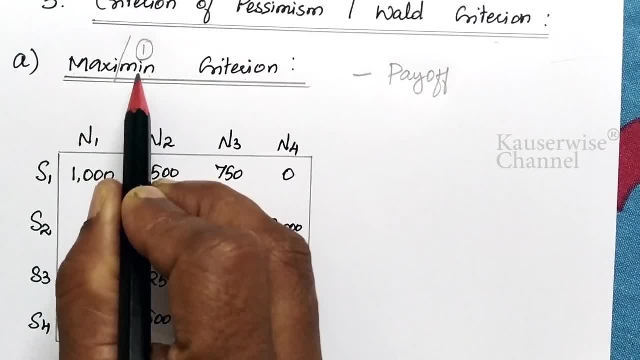 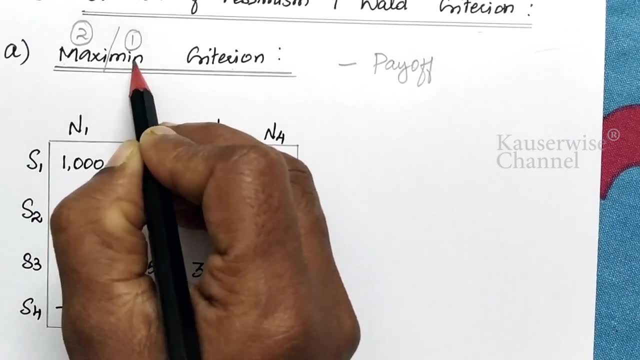 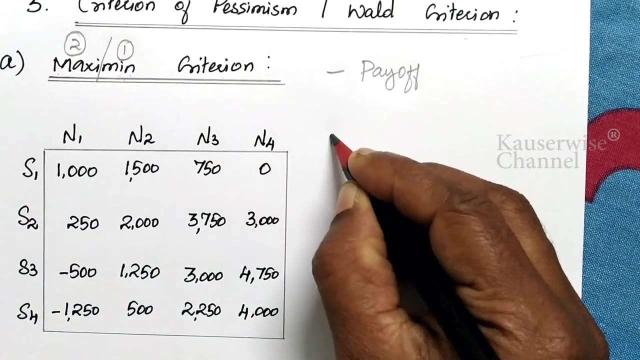 every alternative and after finding the minimum value, then you have to decide based on the first term. okay, first you have to complete the first one, find the minimum value, then you have to take a decision based on the maximum value. i'll show how to calculate so minimum. first you need to find. 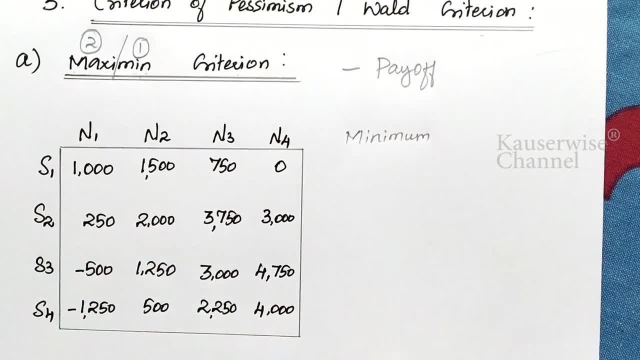 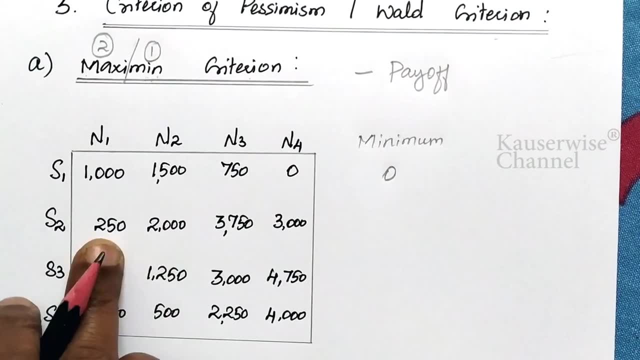 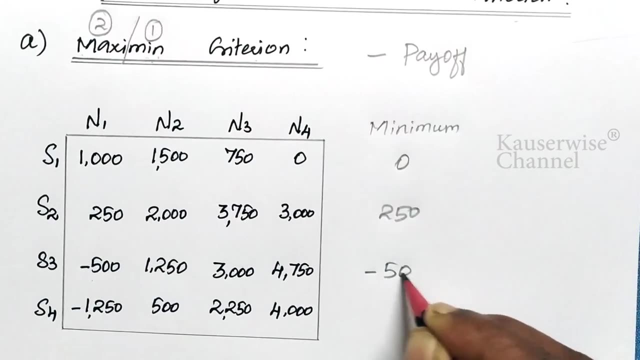 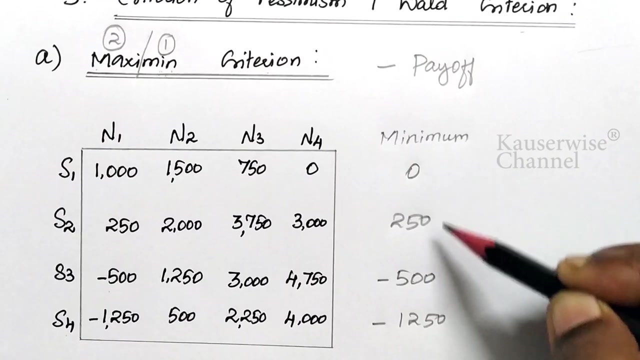 out the minimum of each and every alternatives. for the first alternative minimum value is zero, okay. for the second alternative, minimum value: 250. for the third alternative minimum value: minus 500. for the fourth alternative: minimum value: minus 1250. now, after finding the minimum values for each and every alternatives, now you have to decide. 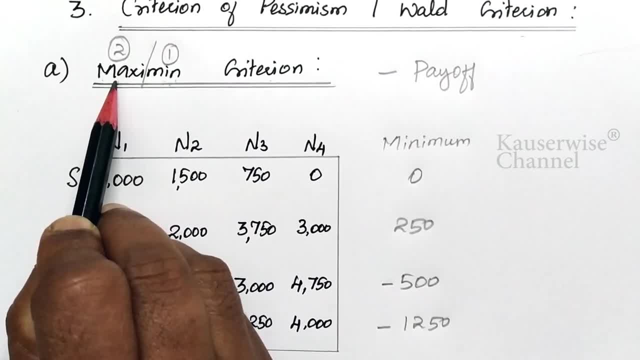 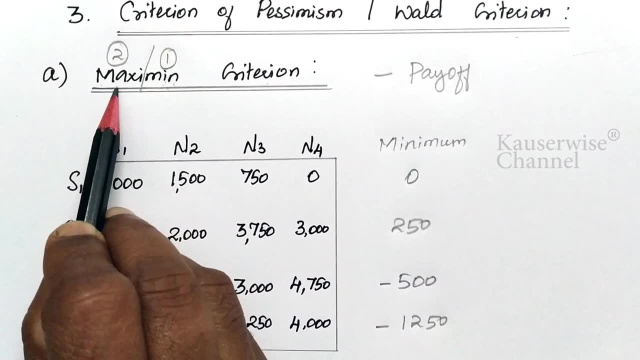 which is the best one. for that you have to select maximum. first we have to calculate minimum, then you have to decide based on the maximum value. this is the first step, and this is the second step. now we have to find out the minimum value of each and every alternative, and then you have to. 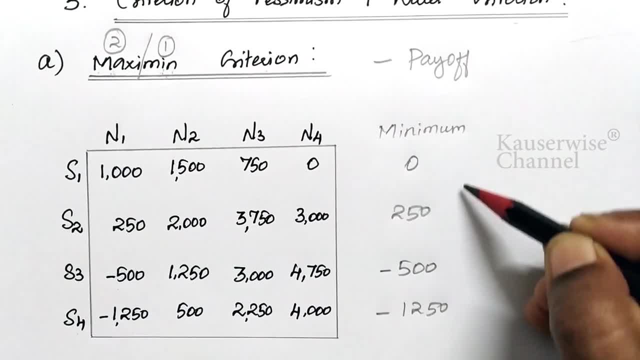 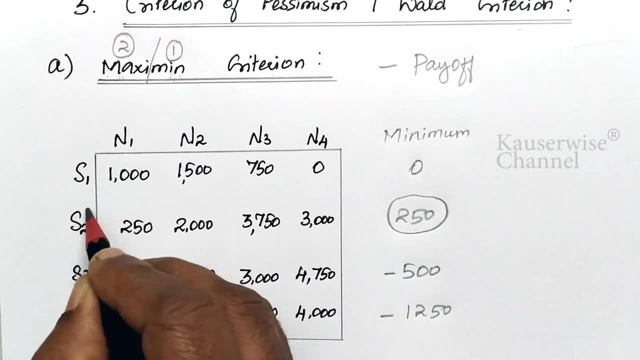 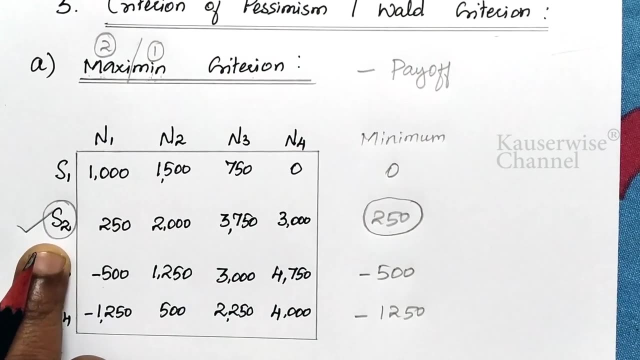 out maximum of minimum value. so now, which is the maximum value out of these minimum values? 250 is the maximum value, so s2 is the best alternative among all other alternatives. so s2 has to be selected as a best alternative for implementation according to maximum criterion. 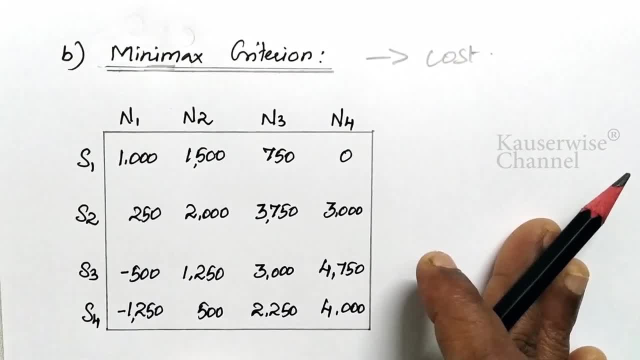 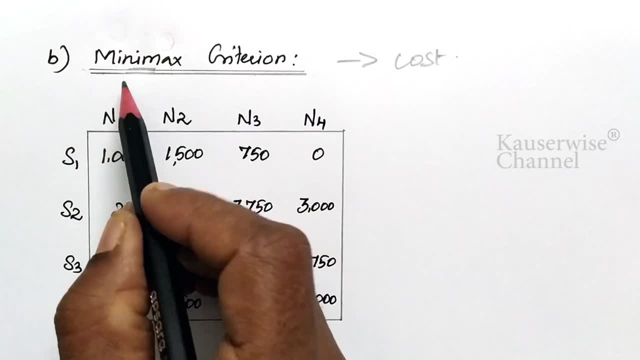 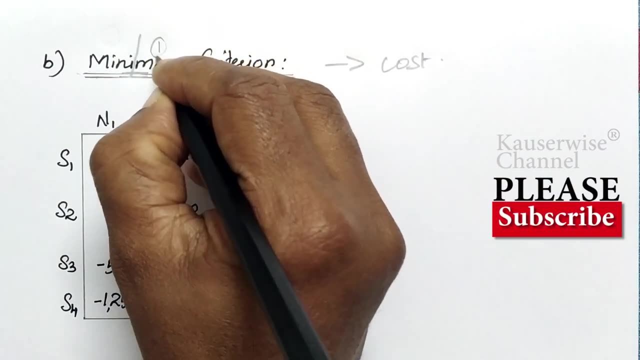 now let us see minimax criterion. okay, so this criterion is applicable for cost matrix. assume this matrix is a cost matrix. now you have to find out maximum value. okay, just divide the term into two parts and first you need to find out the maximum value for each and every. 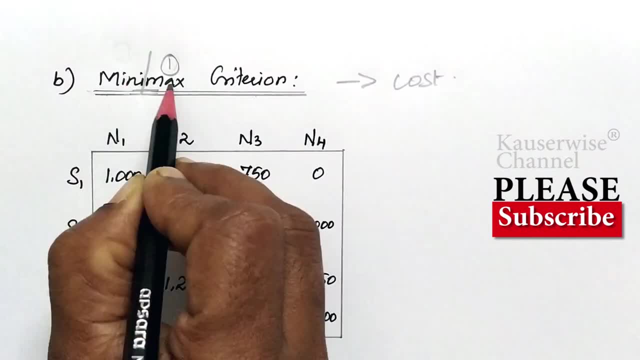 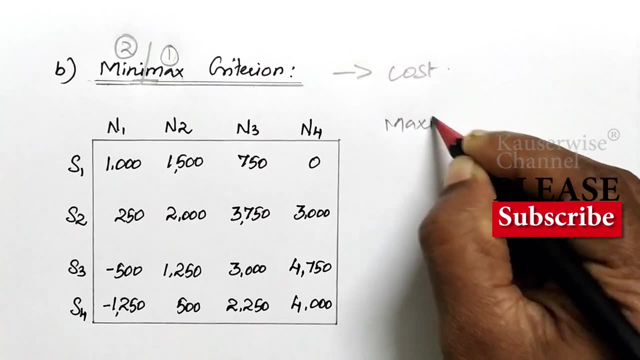 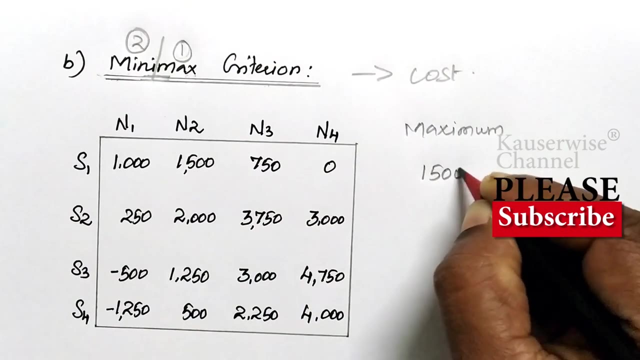 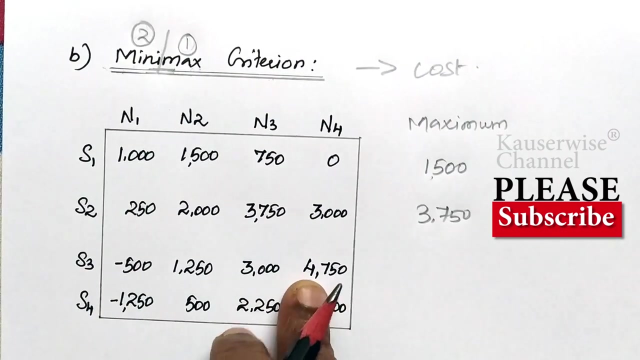 alternatives and then you have to select the minimum of maximum value. so first you have to do the this one that is maximum. find out the maximum values for each and every alternatives. for the first one maximum value is 1500 and for the second alternative 3750, for the third one 4750, for the fourth one 4000. so these are the 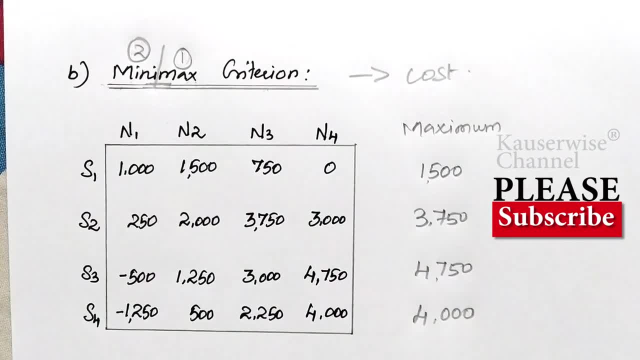 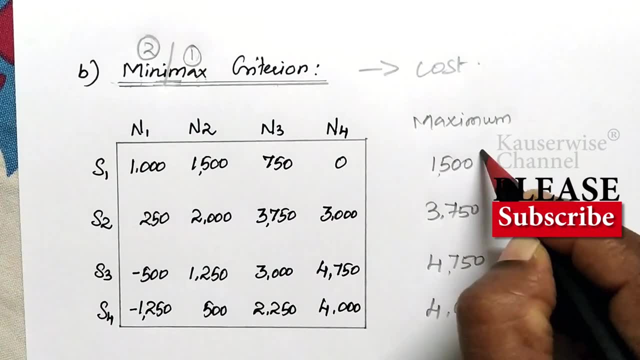 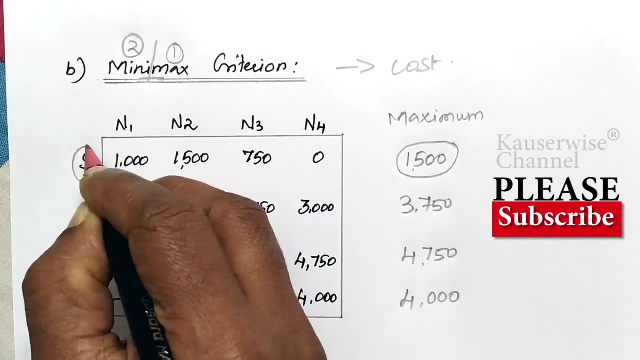 maximum value for each and every alternatives. now you have to select minimum of maximum values. okay, so now which is the minimum value? 1500 is the minimum value. so according to minimax, criterion s2 is the best alternative to be selected for implementation. see according to.